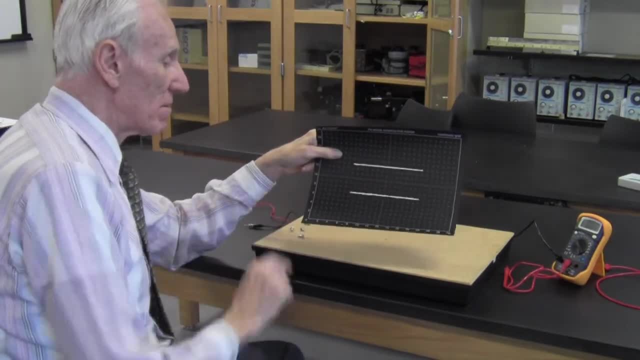 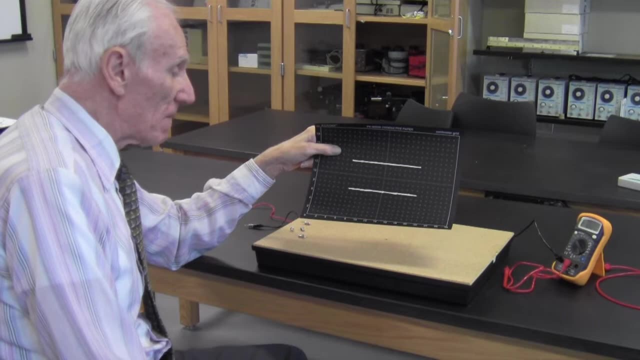 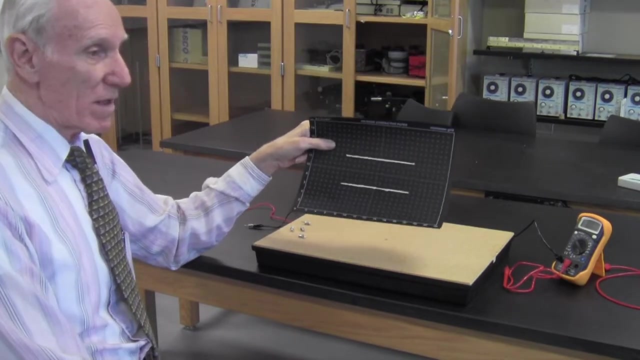 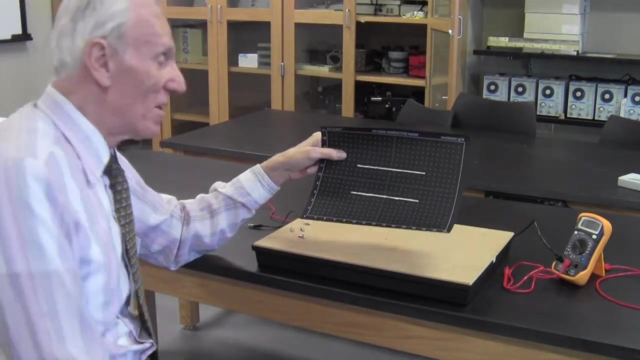 So on this piece of semiconductor paper are drawn two parallel lines with honest-to-goonish silver ink. Every one of these patterns like it's got 50 cents worth of silver on it. But don't go scratching it off and try to sell it. 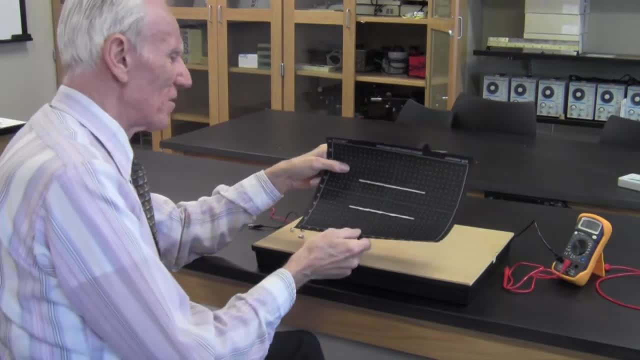 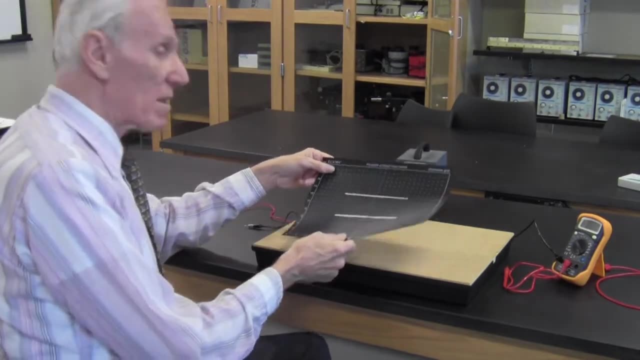 Anyway, well, maybe it's only ten cents, I don't know, but it's, it's got some silver on it, So silver is a really good conductor, like it's one of the better metal conductors, And so it conducts electricity. 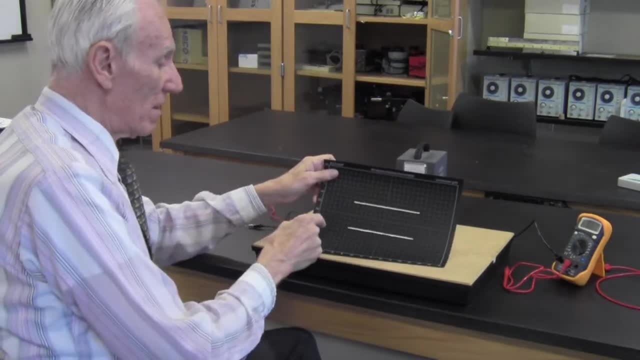 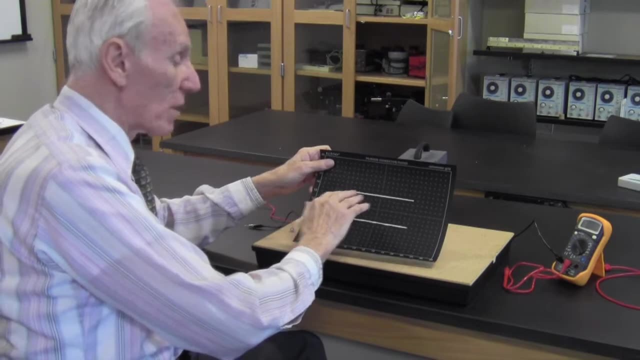 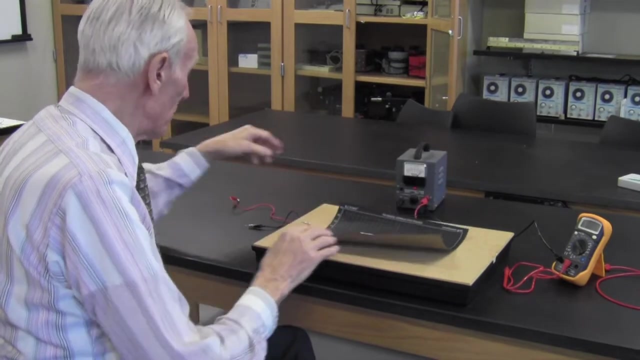 and it can conduct electricity from one side to the other or from the middle to the outside and it can set up an electric potential. We'll get to that later. Electric potential here and another electric potential here. So we have two leads on meters. One's a black lead. 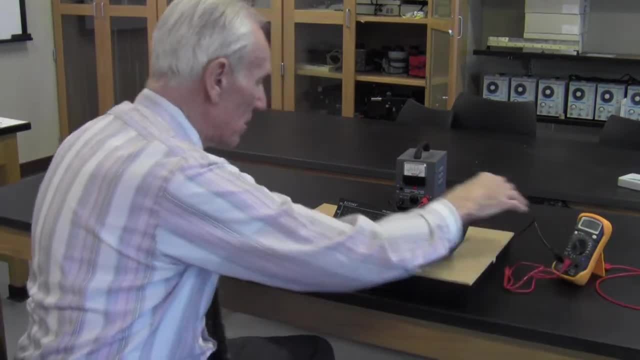 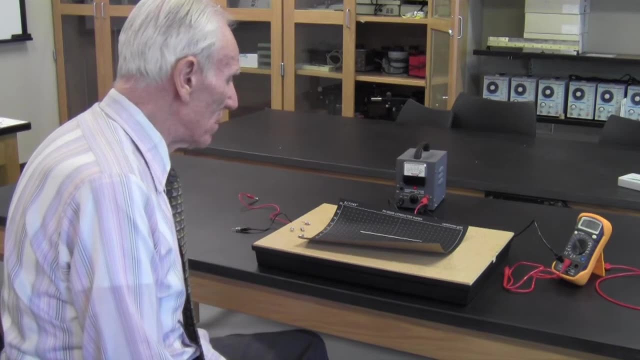 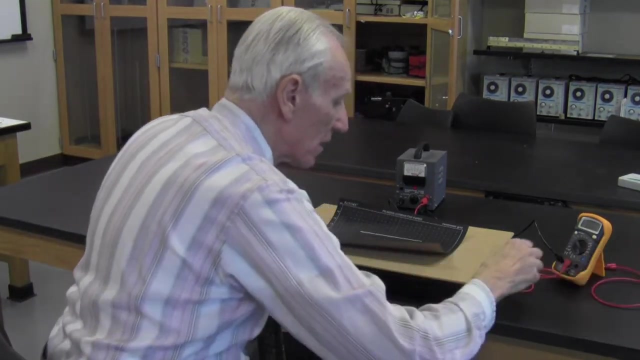 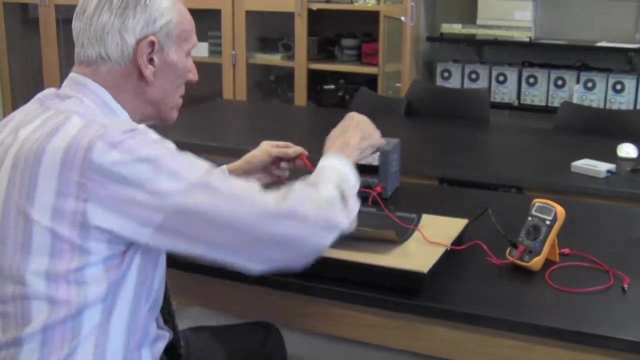 one's a red lead and there's the red lead over here. It's connected to this black lead over here at the power supply, and so we can measure voltages. In fact, I've got this set at roughly six volts, so let's check that out. Okay, it's a little bit high. This is very delicate. I. 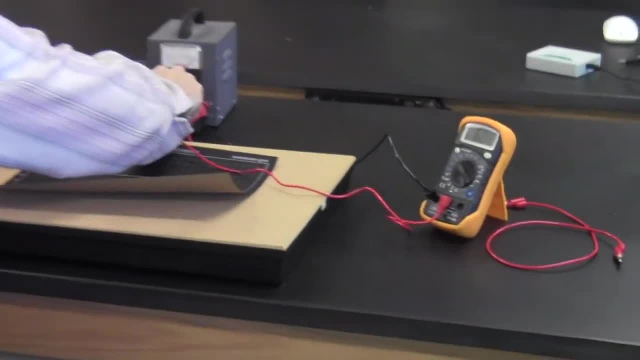 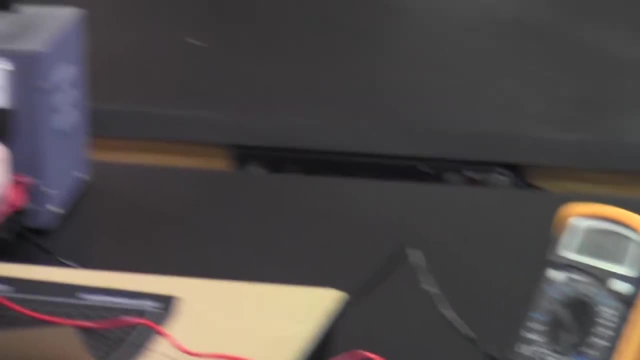 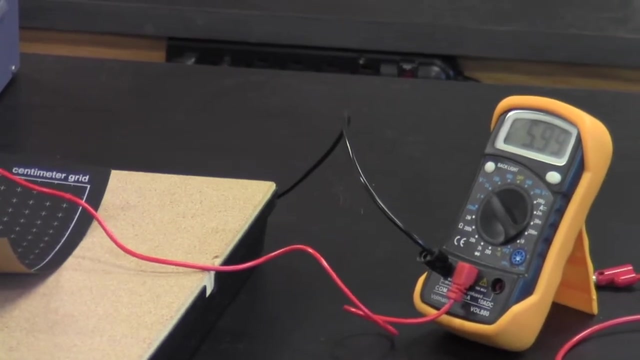 wouldn't mess with this. We're going to try to set this for you so that it stays at six, So I can turn this down just a little bit. So it's closer to six. Oh, that's close enough. Okay, that's six volts. 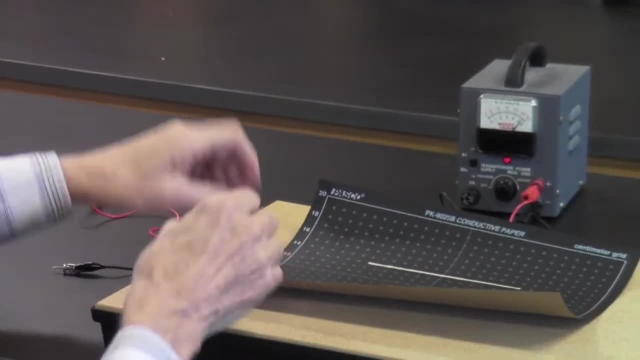 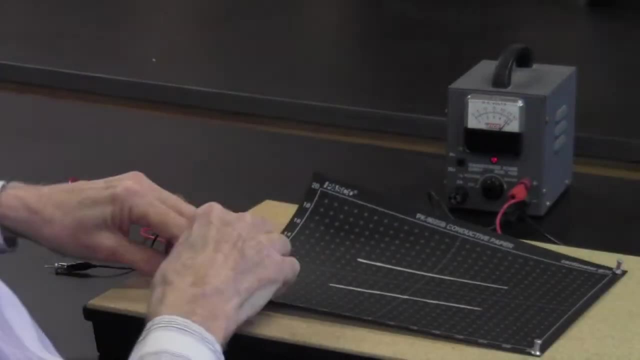 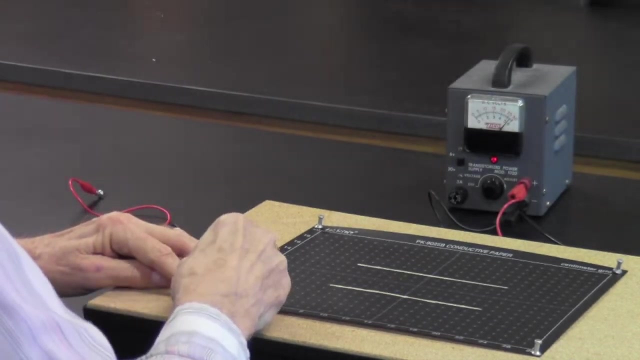 So I'm going to connect this red. First of all, I'm going to pin this down so it's not so curled up and stays nice and flat. for my experiment, These are metal push pins, which means they're conductors and they will transmit the voltage. 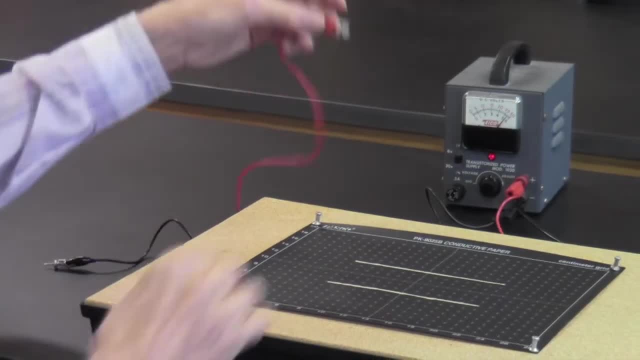 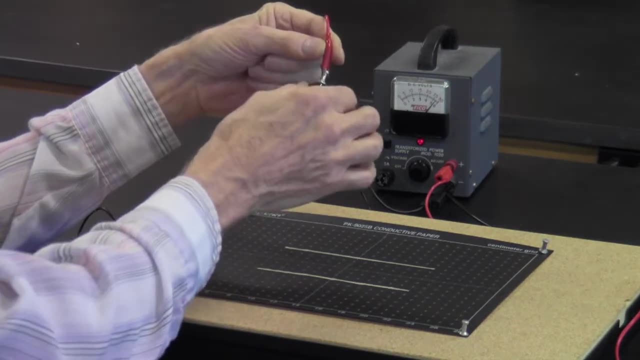 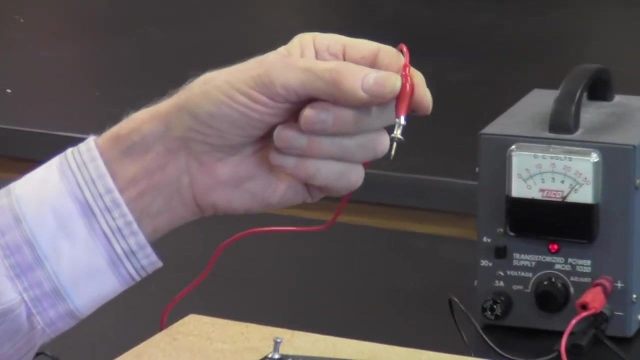 or they'll carry the voltage to wherever we put this. So I've got these pins, I've got these little clips here on these pins so that they're like in the same direction as the pin itself. and the reason for that is- you'll learn later, as I mentioned earlier, that the electric fields 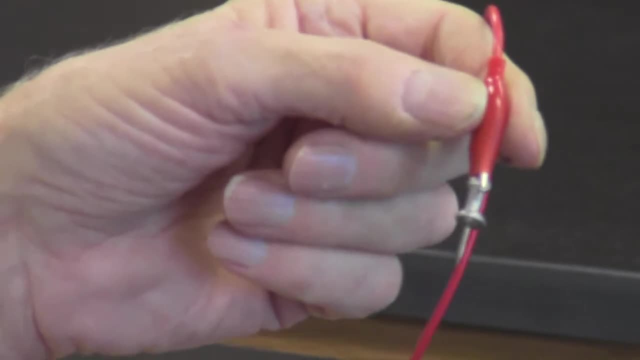 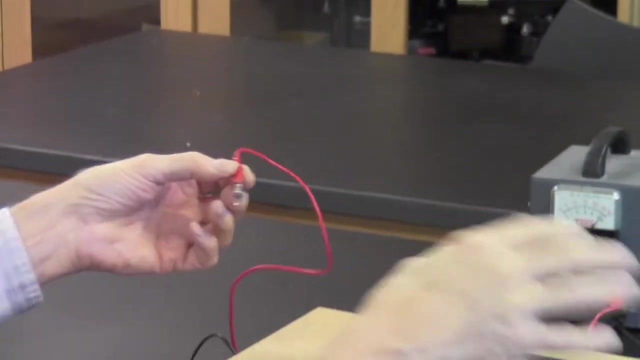 can be set up by single charges, like we talked about for Coulomb's law, or they can be set up by a whole bunch of charges. There's a whole bunch of charges in this wire which recibies the cables just like it would any product be spread out. 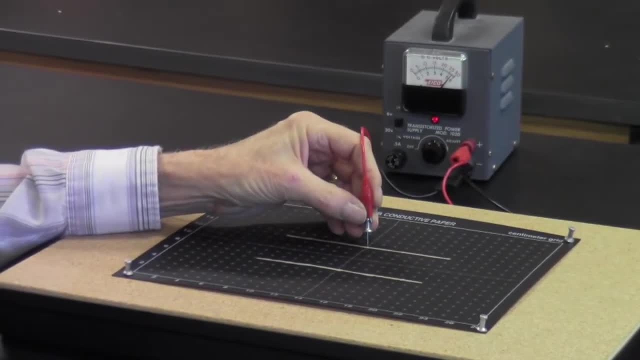 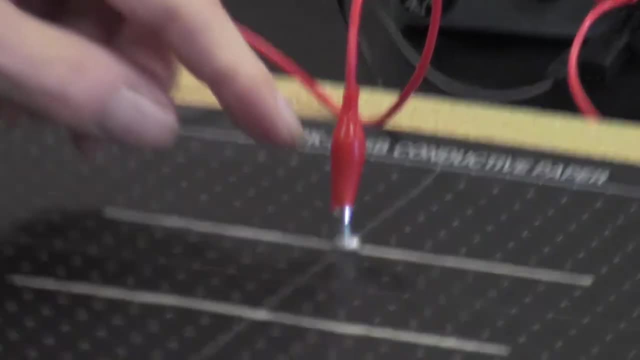 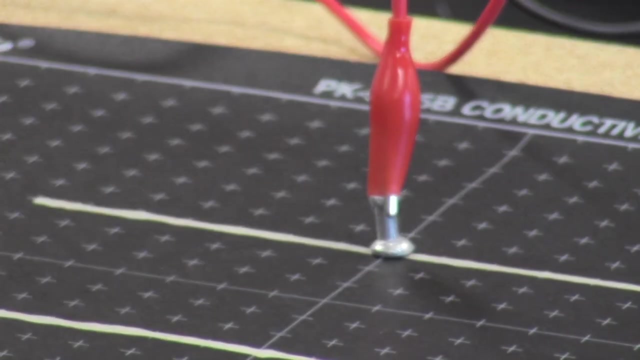 And they're put there by this voltage supply which pushes the charges in the wire. so I'm going to connect very carefully this wire 2 with this push pin and I push it fairly hard so that it makes a good electrical contact with that silver line. 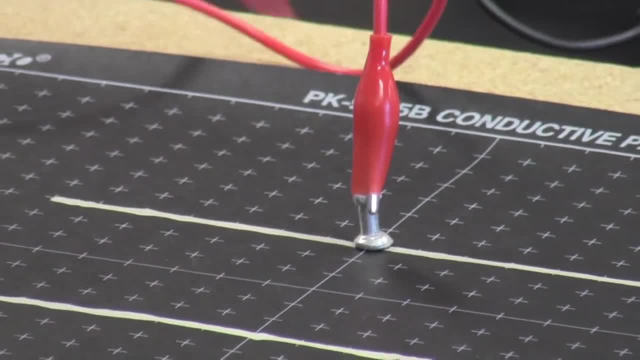 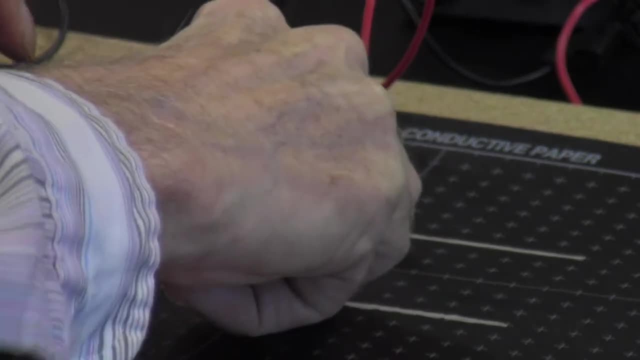 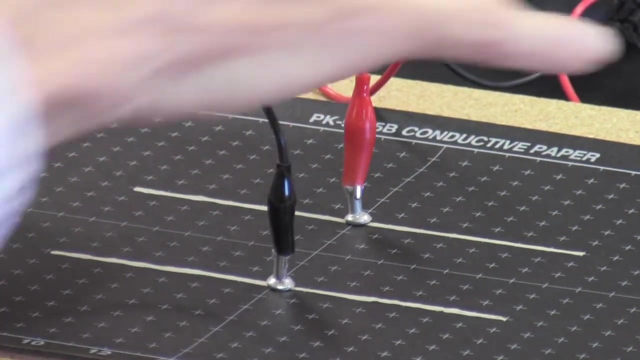 to be connected to the other line And I'm going to push it down so that it's nice and flat. There is an electric field set up by these wires And I really don't want to have it mess with the electric field set up on this pattern here. 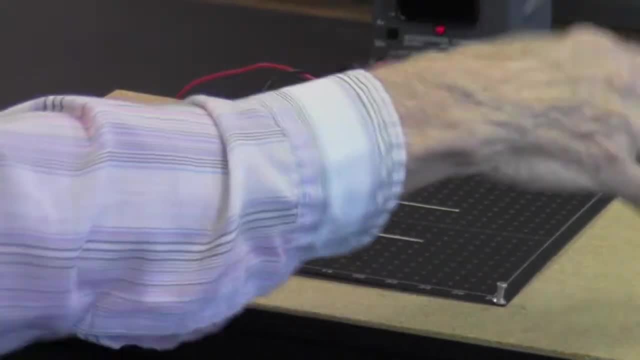 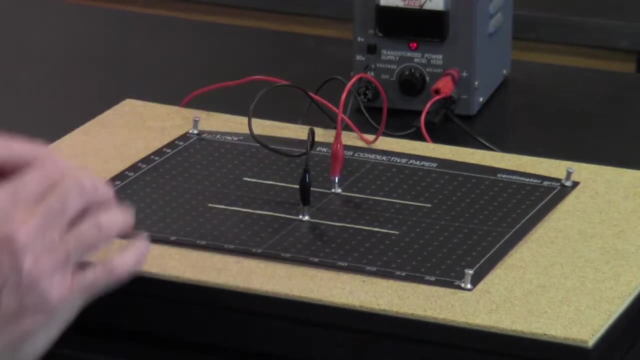 This is kind of like a two-dimensional electric field. So I'm getting those wires away from the pattern. That's why I've got them hooked up that way, so they're not resting on the pattern. So I don't want the electric field of that wire. 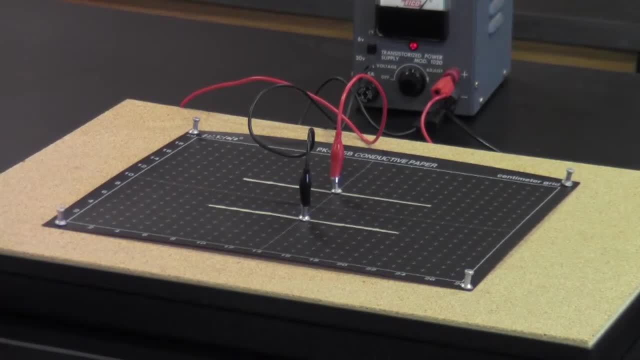 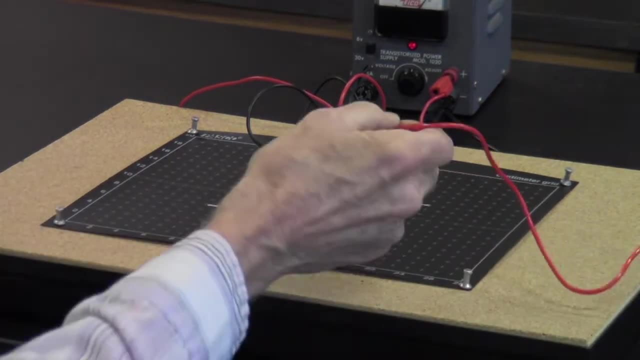 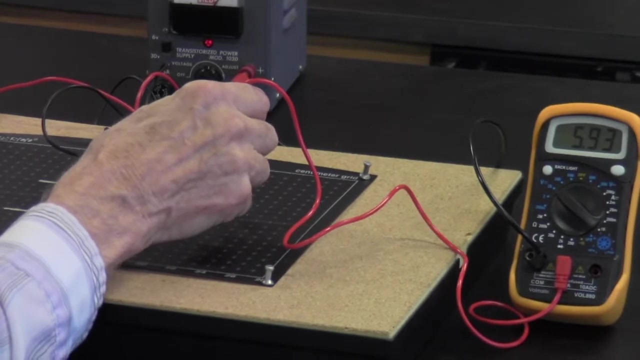 to be fighting the electric field on this pattern. OK, so I've got them all hooked up And if I look over here at this, take a look at the meter. look over here on this. It's almost 6 volts here. 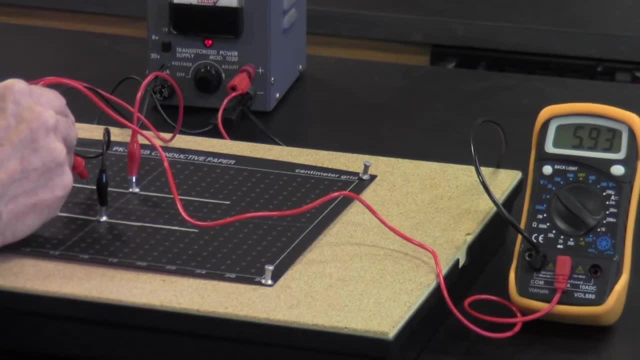 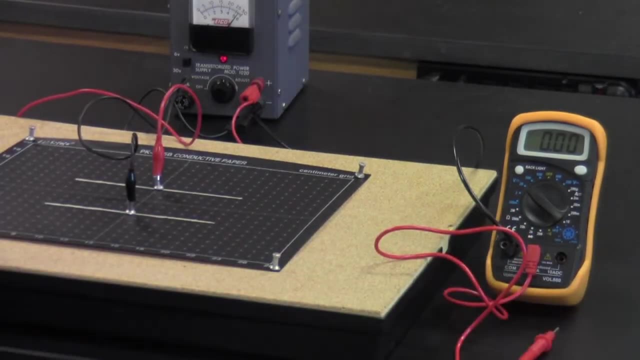 It's 6 volts here, 5.93, 6 volts. here It's 5.93, 5.93.. It's 5.93 all the way from the left to the right end of that pattern, of that line. 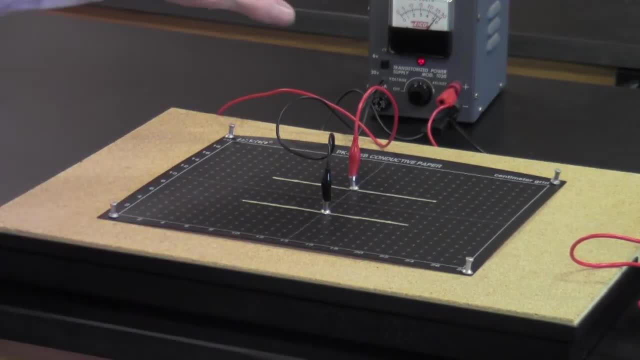 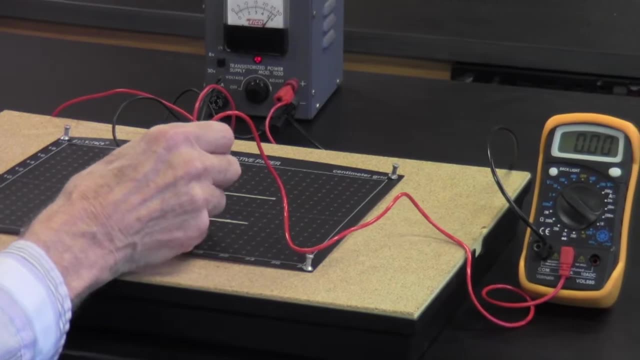 that silver line. And again, I guess the meters changed a little bit so it was closer to 6. But it's 5.93.. And over on this side the voltage is 0, or almost 0. It's not quite 0 on the ends. 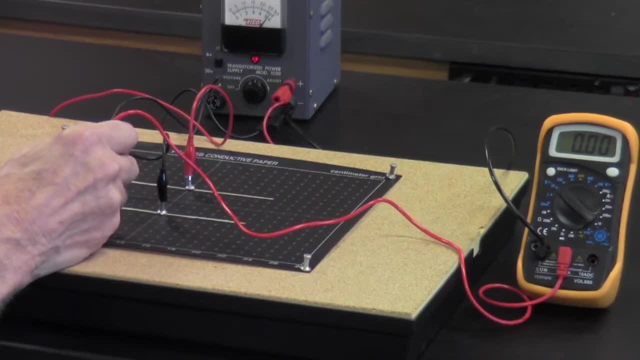 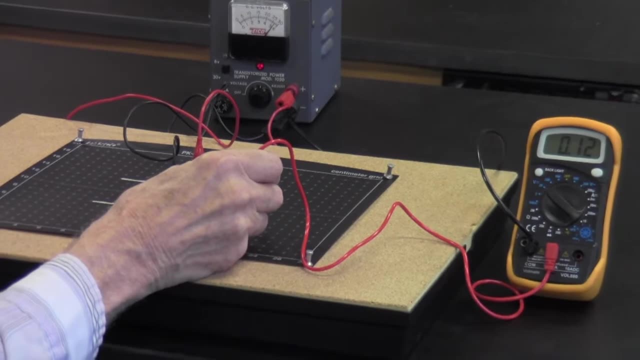 It's almost 0.. It's close enough to 0 to call it 0.. OK, so on this end it's a little bit, not quite 0.. OK, where are, if you? it's pretty much 0 everywhere. 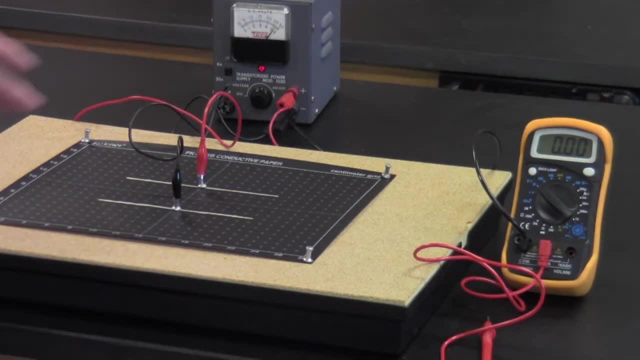 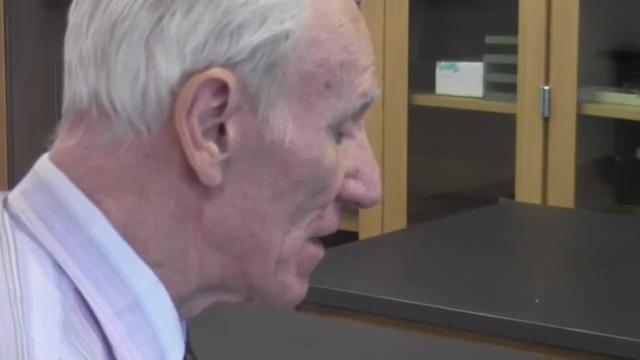 OK, so this is called the 0-volt line And this is the 6-volt line And we call them equal potential lines, equal potential lines, equal potential lines because they have the same potential, the same voltage. Those are not quite interchangeable. 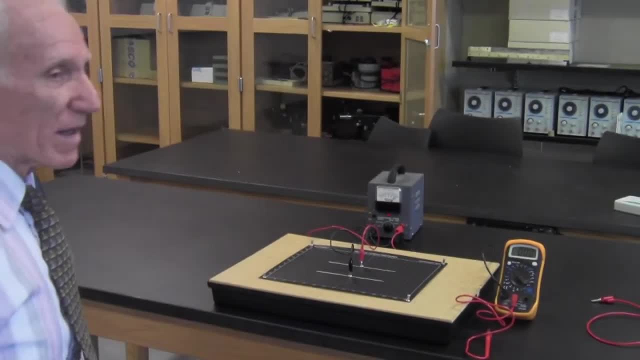 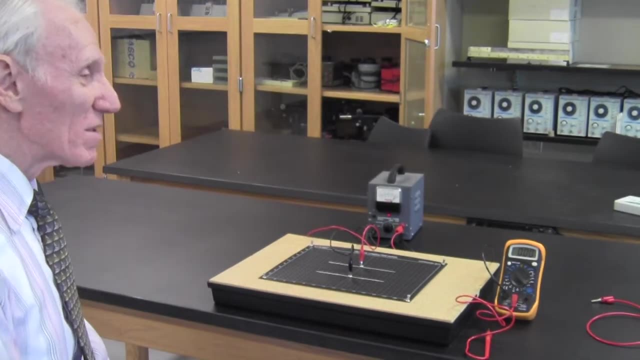 The same voltage is 0 on this line and 6 on that line. This is a semi-quantitative experiment, So you can't get too too fussy about. oh, is it 6.03, or is it 5.3,, 5.92, or what? 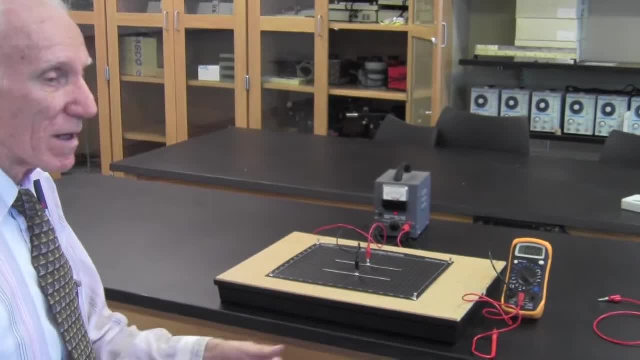 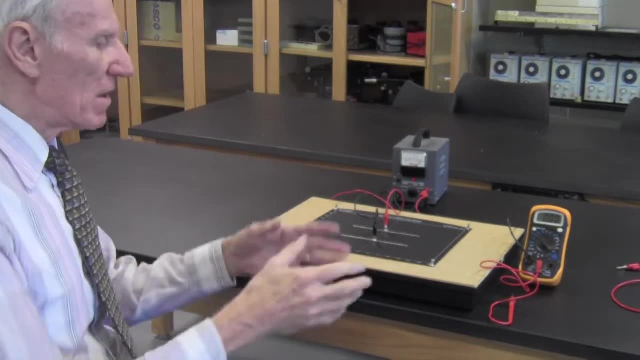 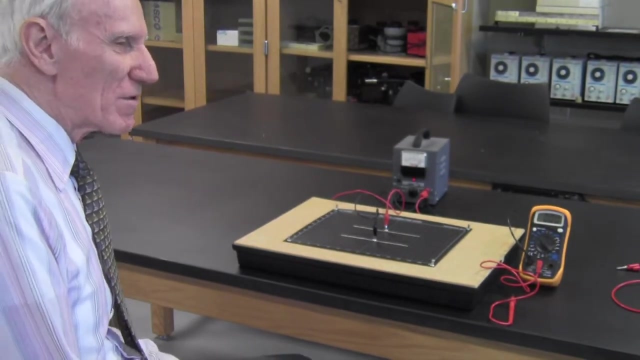 It's 6 volts, give or take a little bit, but not much. OK. so we're going to be drawing some lines here and measuring some values And they're kind of crude, So you can't really do a sophisticated error analysis. 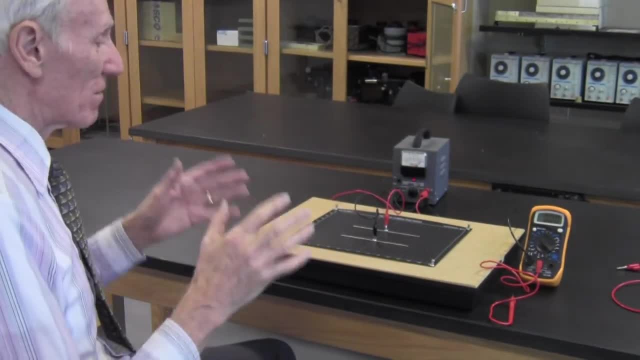 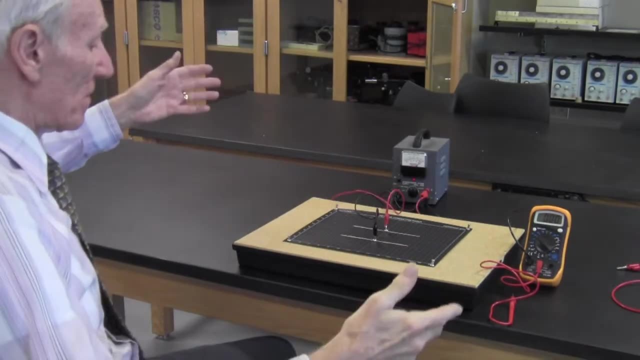 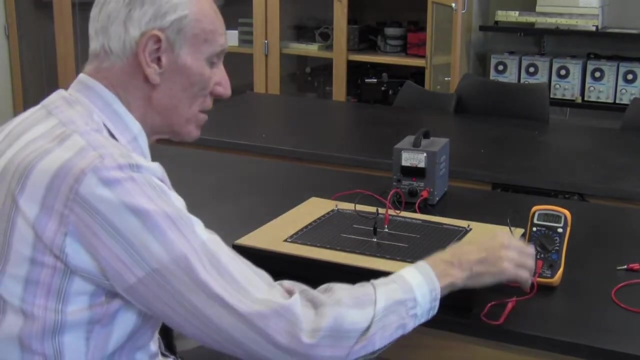 here because it's a semi-quantitative experiment, But that's OK for once. So I have set up, everywhere in space, everywhere in the universe, an electric field that's emanating from these two lines. Now my job, your job, is to measure the locations. 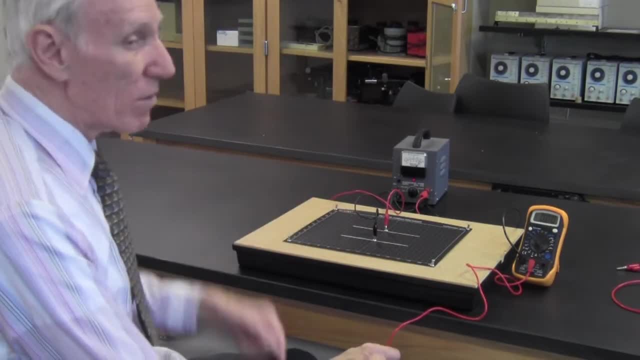 in the electric field. We've already done the 6-volt line and a 0-volt equal potential line. Your job is to find the 1,, 2,, 3,, 4, and 5-volt potential. OK. 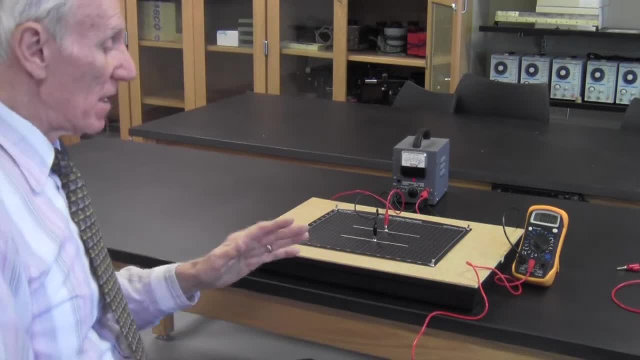 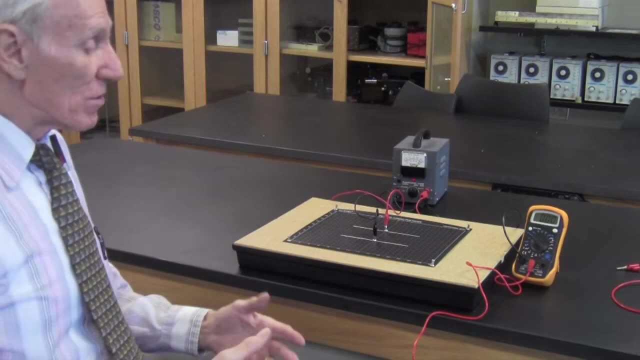 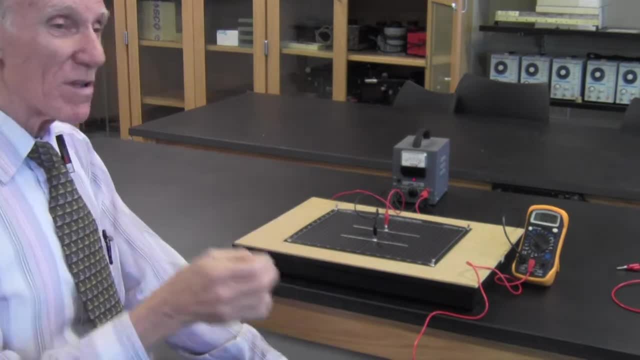 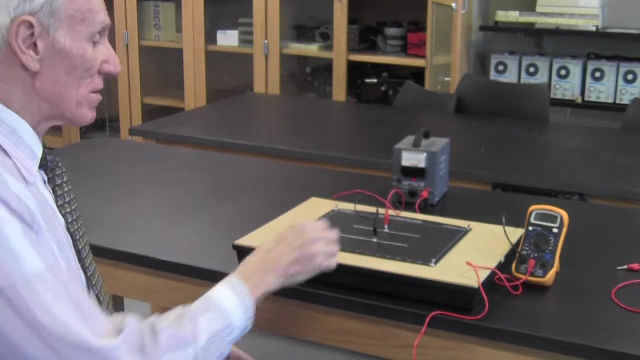 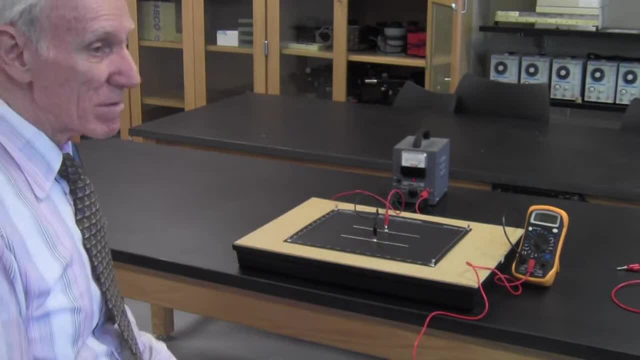 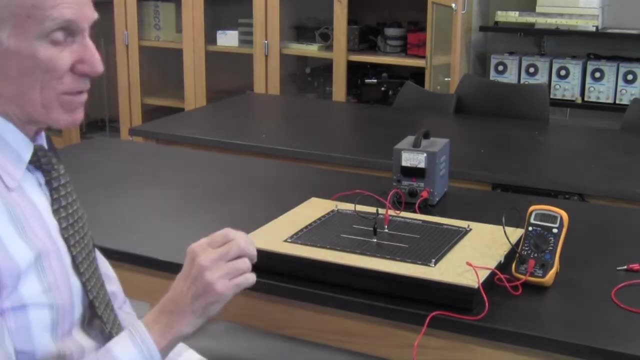 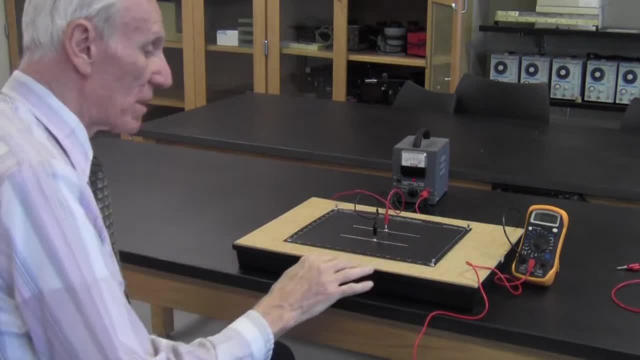 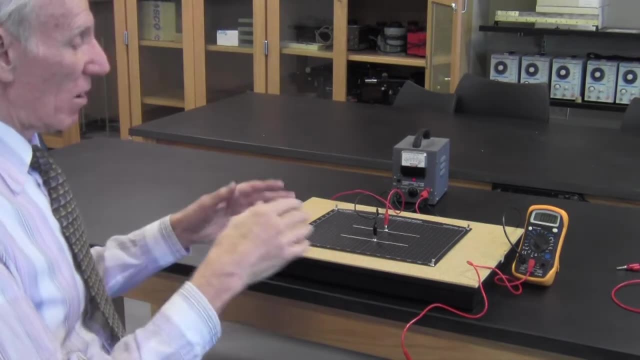 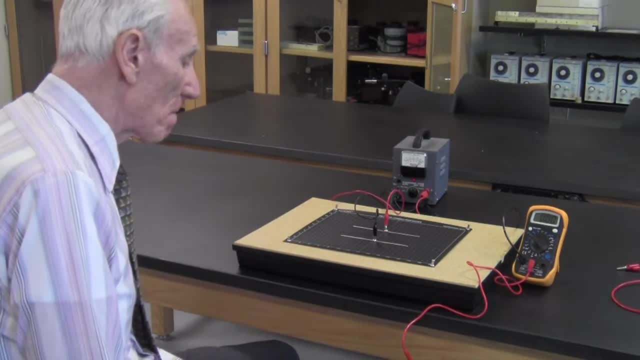 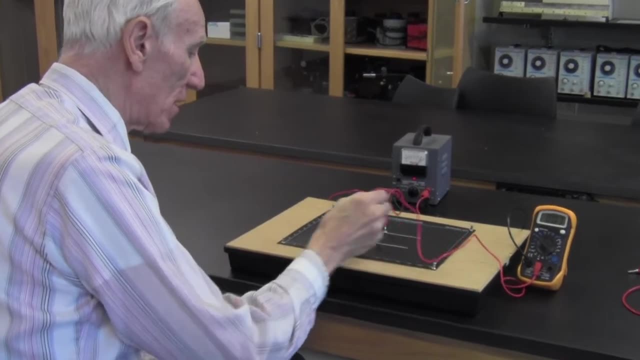 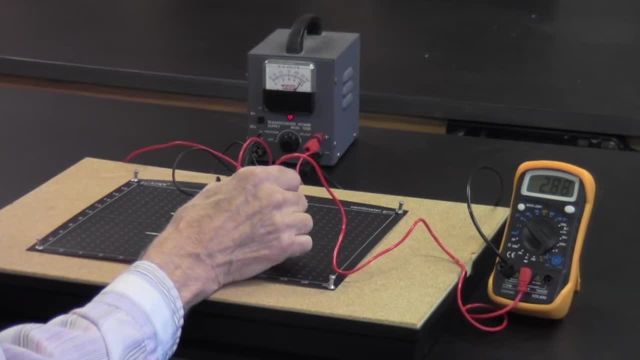 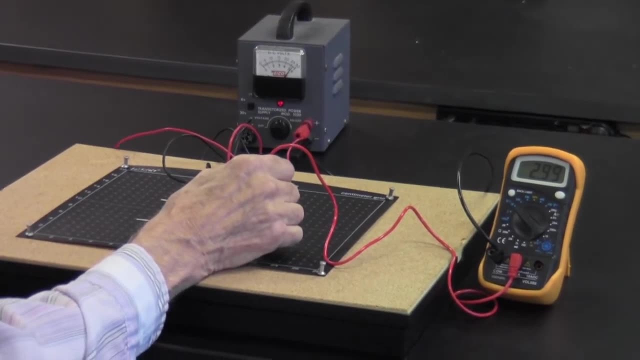 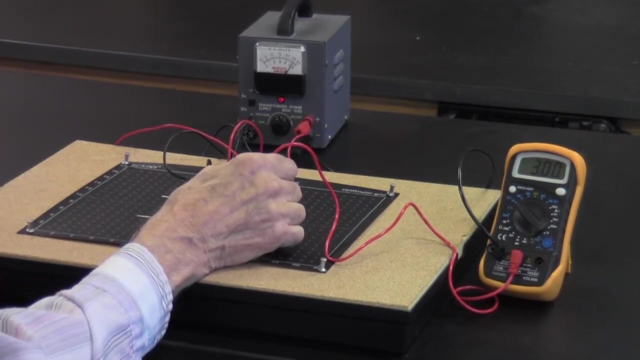 So somewhere in the middle it ought to be about three volts. Oh, and let me move that. OK, There it is. It's- surprisingly- or not surprisingly- exactly in the middle, because three is exactly in the middle between zero and six. So there's three volts. 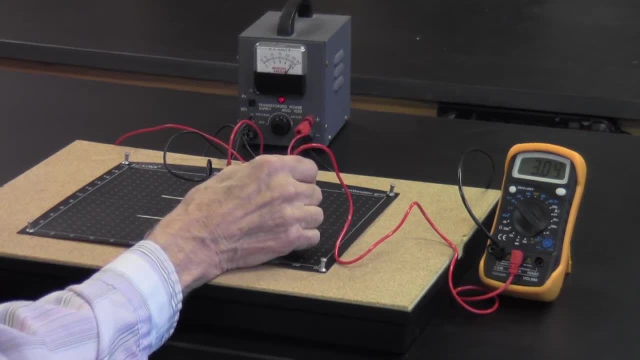 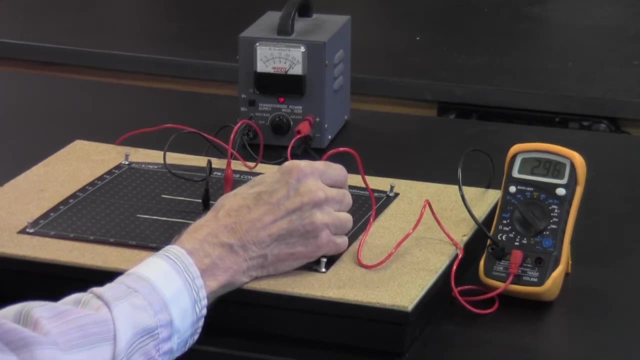 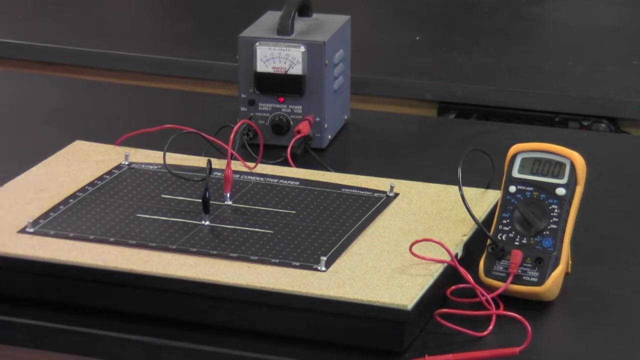 So I'm going to find another three volt point and I'll put a dot there. and I'll find a three-volt point here and put a dot here and you'll find, probably, depending on the quality of the pattern, that that line basically goes straight across or pretty much straight across. So put a. 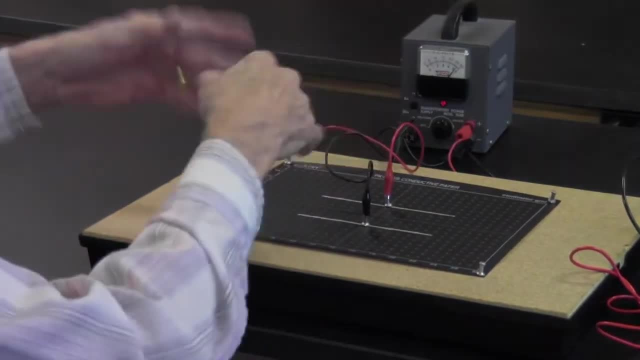 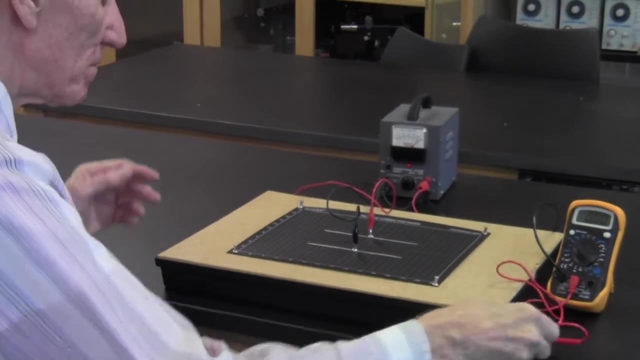 bunch of dots here, you know 12,, 15,, 20, whatever dots. just what we just did, what I just did, and put a dot where the probe is touching the paper and then connect those dots Again. that's called an equipotential line and that's. 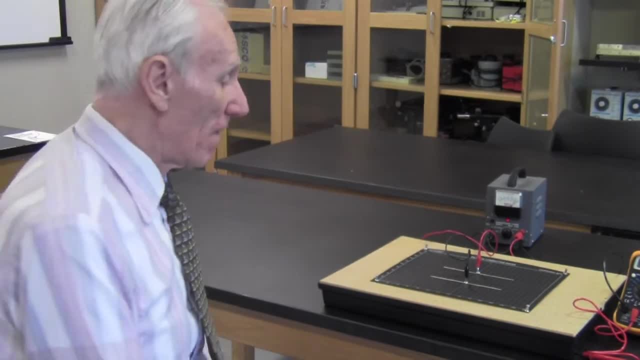 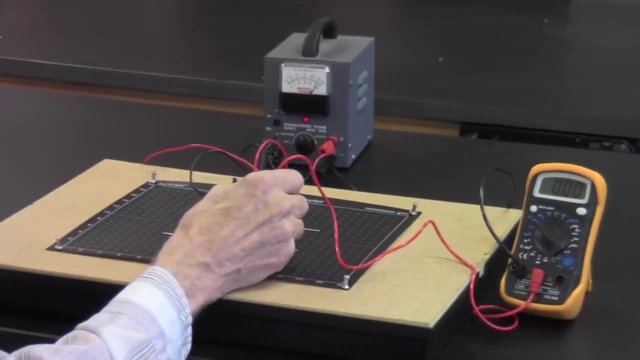 the three-volt equipotential line. Okay, let's take a look at the two-volt line, for instance. So the two-volt line ought to be closer to the zero-volt equipotential line. It's going to be over here someplace and there it is. It's. 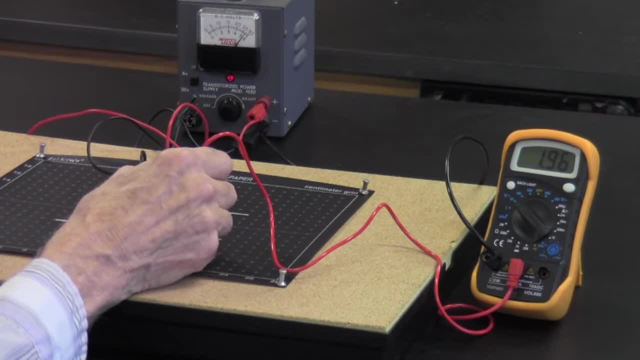 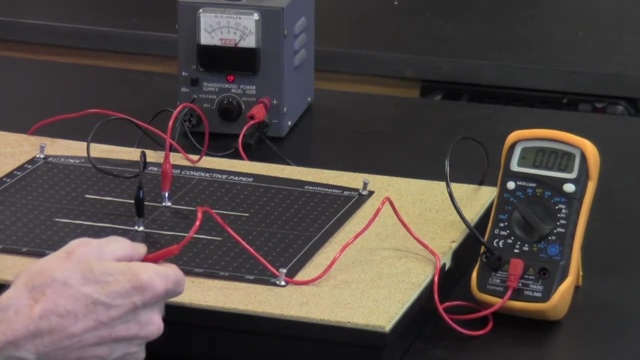 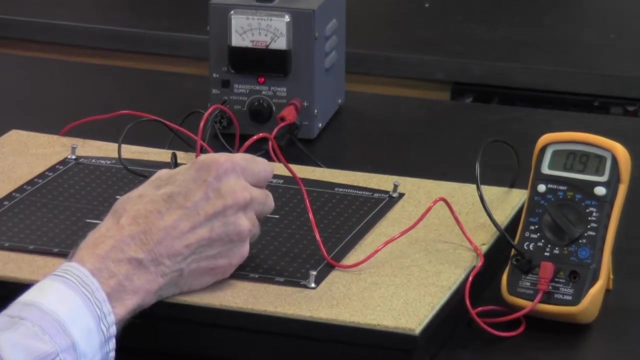 pretty much. I've kind of planned it this way, that is, these two lines are six centimeters apart and we've got six volts here, so it's about one volt per centimeter, right. So every centimeter here's the one-volt line. it's at one centimeter There's a two-volt. 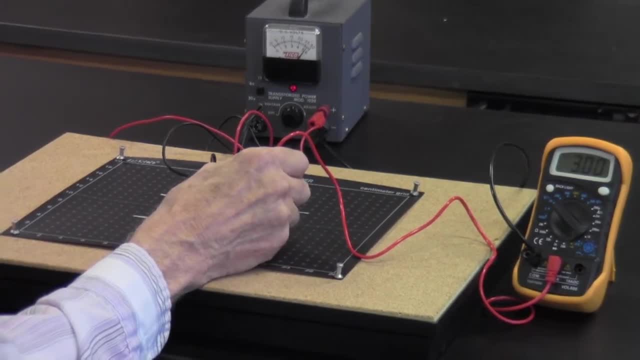 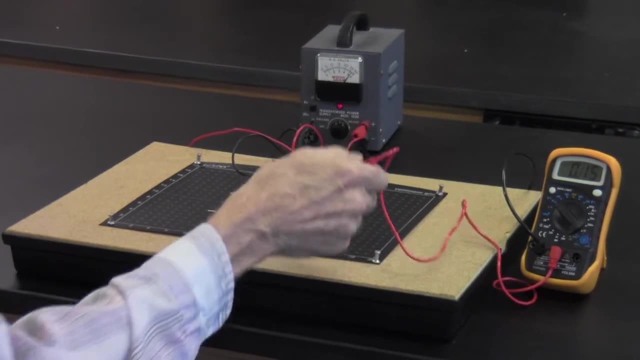 line: it's at two centimeters. There's a three-volt line. we already saw that that's three centimeters. There's a four-volt line: it's at four centimeters. There's a five-volt line: it's at five centimeters. No surprise, right? So what you're going. 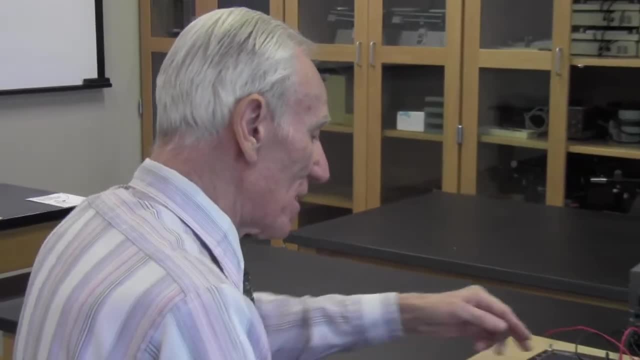 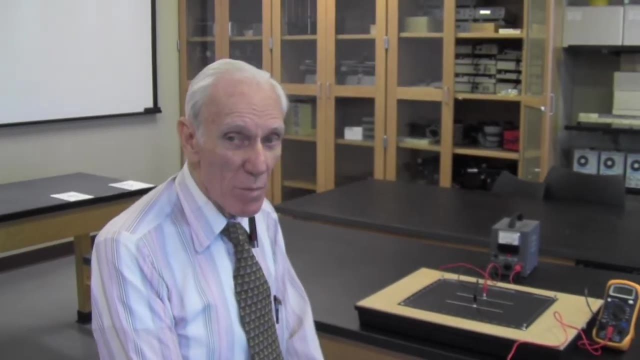 to get here- and I'm not going to tell you what you're going to get elsewhere, but what you're going to get here- and between these two lines are five parallel lines, essentially one centimeter apart, And we want to talk about that a little bit later. in terms of how do you? 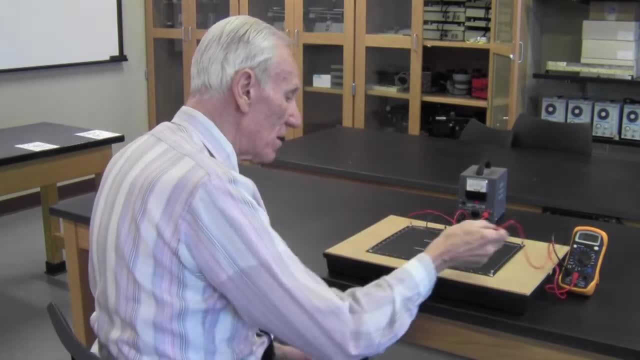 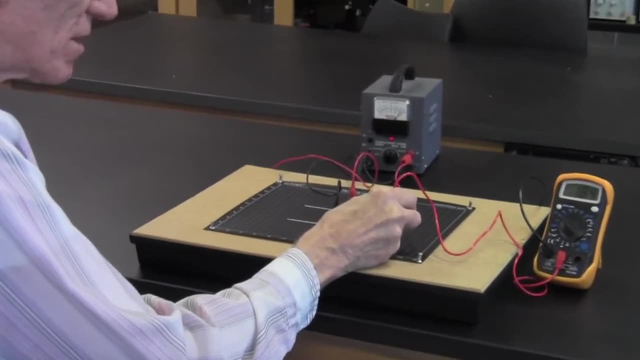 analyze this, So, but then when it comes out here, let's look for the two-volt line here. So two-volt line, I just keep poking around until I find the two-volt line and I'm getting warmer and getting warmer, almost there. 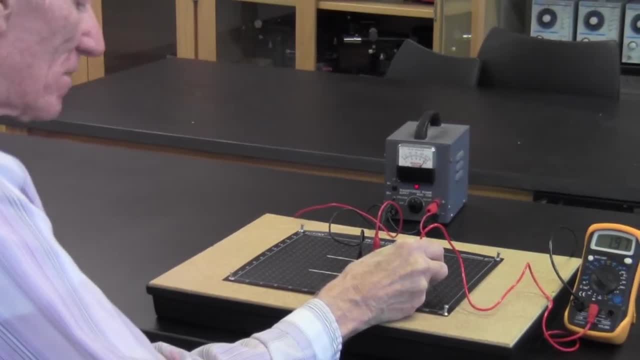 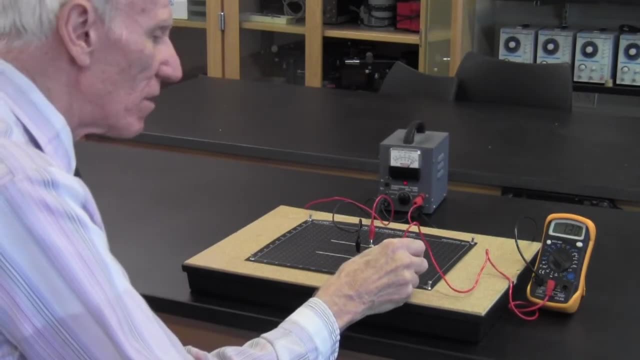 Okay, there's a two-volt point and it's kind of it's going away from this two second line here. it's going out this way. So you want to look for that two-volt line. everywhere There's got to be a two-volt. 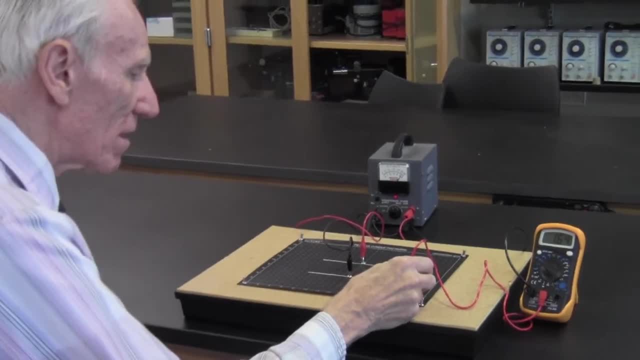 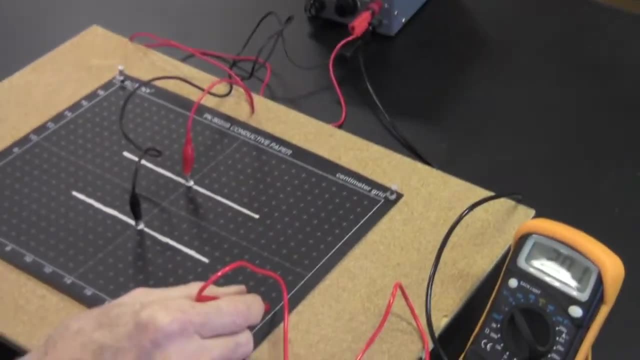 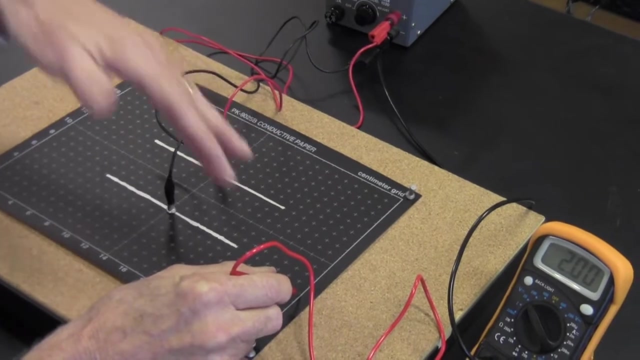 line out here someplace. Okay, there it is. The two-volt line is way out there. So trace the two-volt line all the way from this, like this white border. from one side all the way across to the other side, There's a two-volt line. 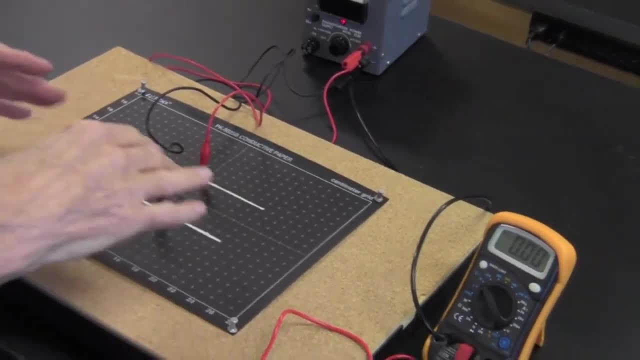 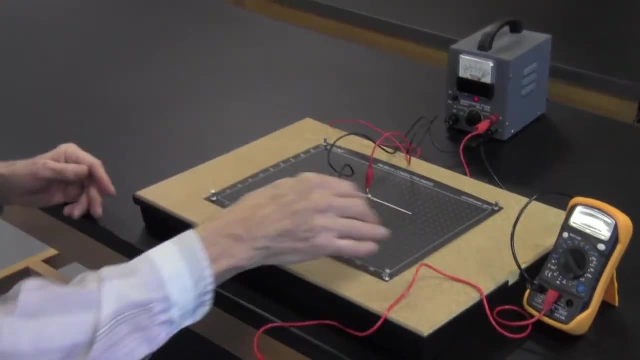 Right over there. Okay, two-volt point. So put little dots there and draw that. Don't draw the line in, because if you start smudging this, if you start drawing lines with the chalk marks and chalk lines, you're going to get it all. 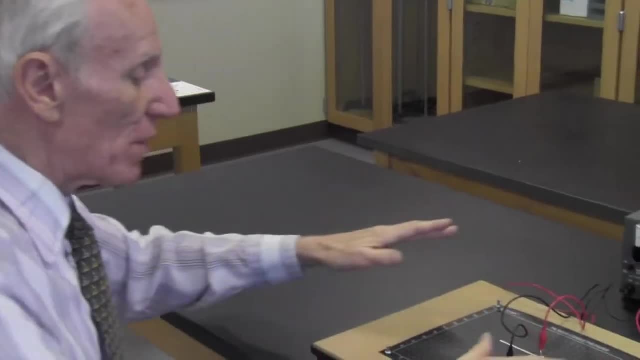 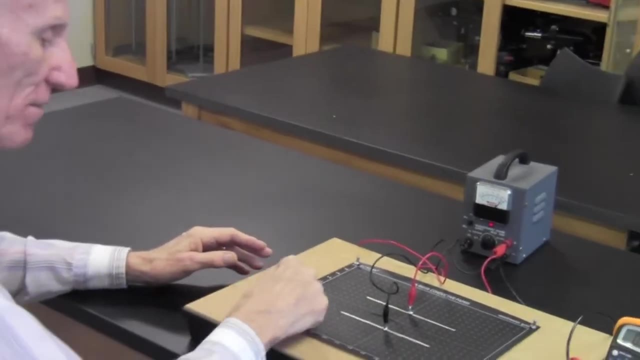 smudged up. So we're going to, we're going to- produce this pattern and take it off, take the leads away and then, with a piece of chalk, draw a line from one side to the other. that marked the two-volt potential, equal potential line. 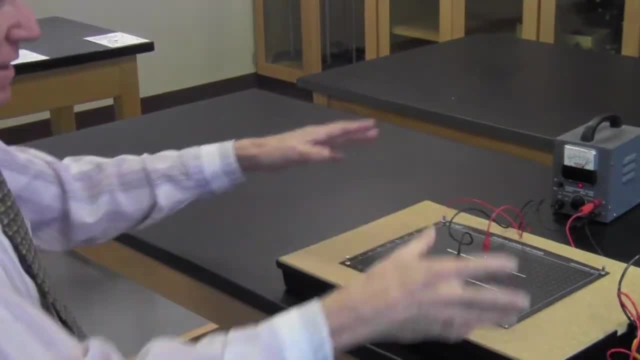 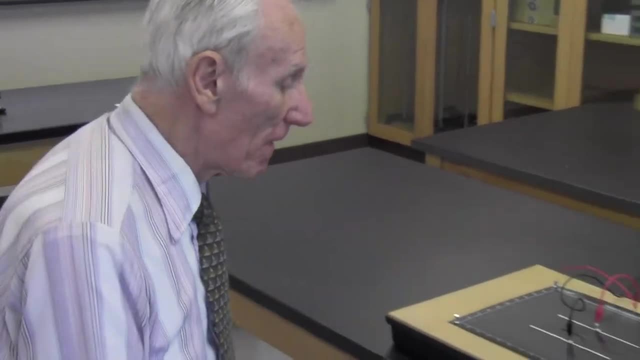 And the three-volt, and the four-volt, and the five-volt and the one-volt. So you get a pattern And we have to talk about: what do you do with that pattern? How do you get the electric field out of that pattern? Okay, and then we'll do one with: 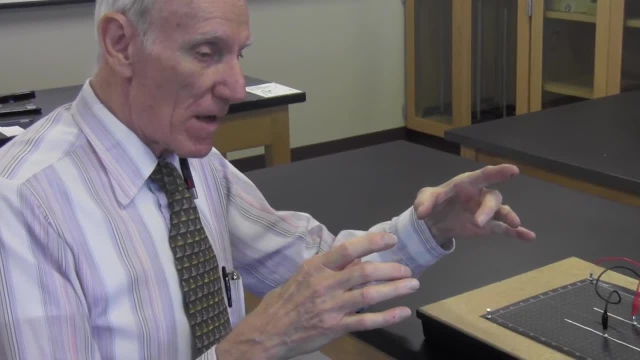 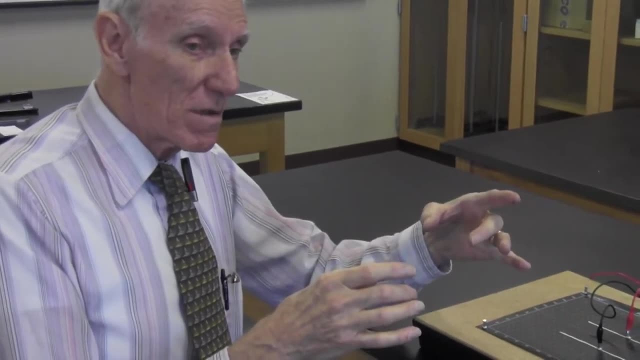 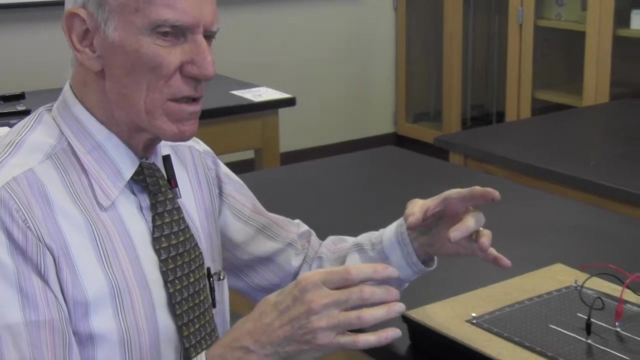 two circles And I want you to especially measure the voltage inside, inside of those two circles and make a note of that and think about what that means. You may not understand really well what that means until we get to the chapter on electric fields and electric potentials and 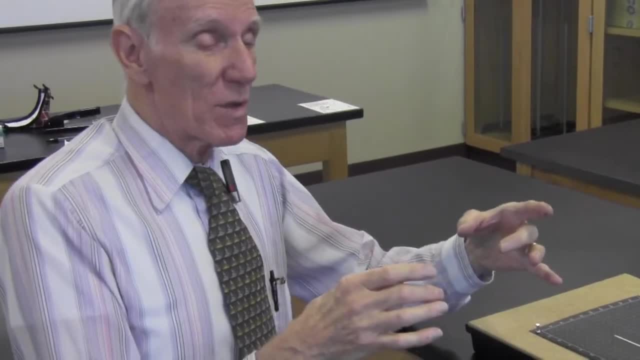 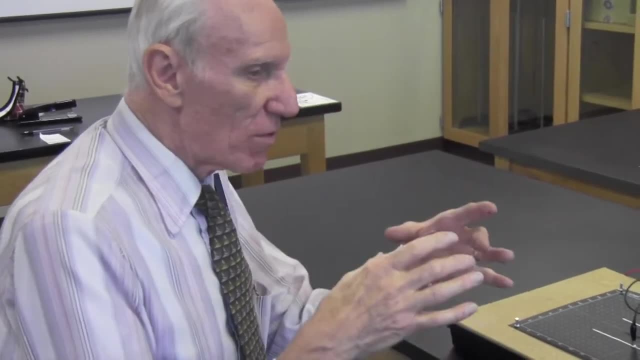 things like that. But see what you get experimentally and if you don't know quite what to make of it, at least report what you get experimentally, So that what's the voltage inside of each of those circles, And you'll hook them up. 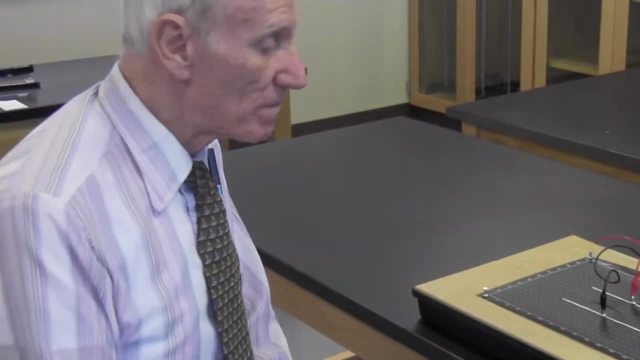 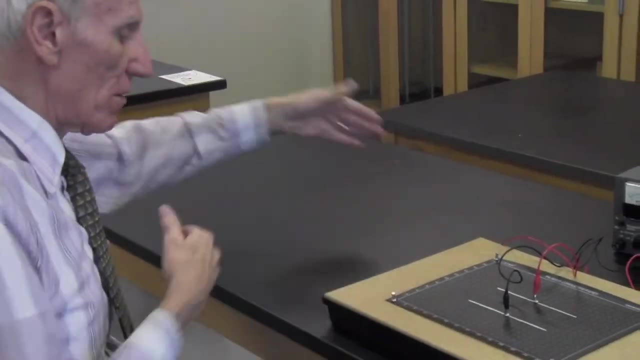 like this: one wire to one circle, one wire to the other circle. Okay, so I'm not going to fill out this pattern, but you can see that the lines kind of diverge as they go out here and they go out here and you want to look for lines everywhere. 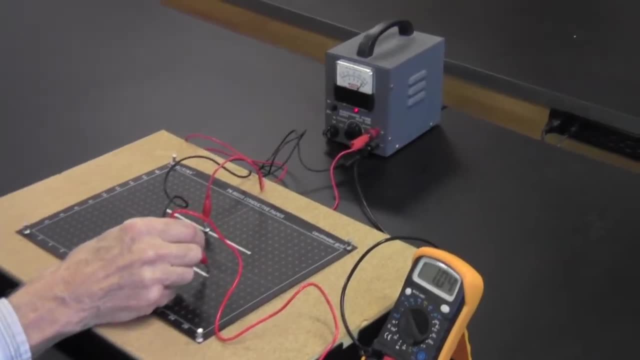 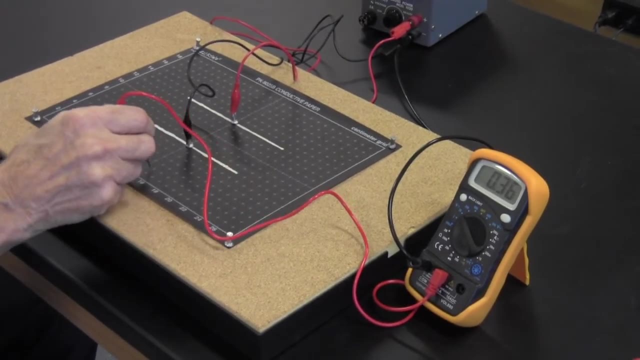 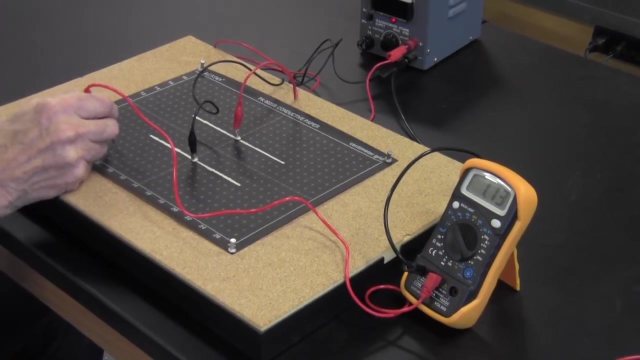 So here's a: here's a one-volt line here, there's a one-volt line out here, someplace like here, and there's no one-volt lines in here until I get over to here and there's another one-volt line. Okay, so that one-volt line kind of. 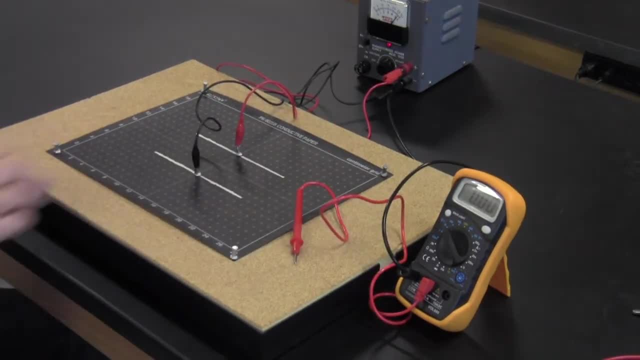 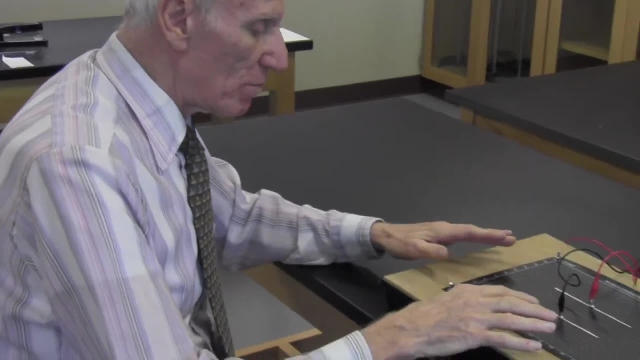 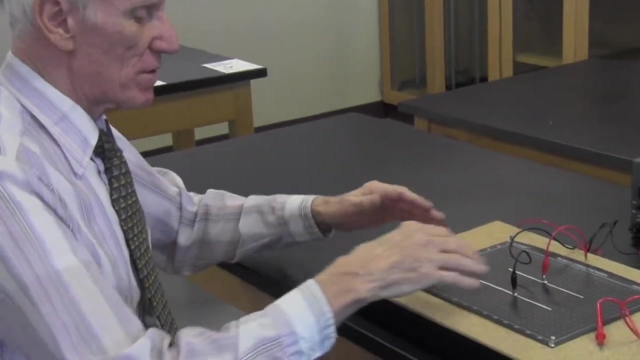 wraps around a little bit. Okay, so that's that's the way you do this experiment, and finish up all all five lines. if, if they, if they start to get kind of confusing, Maybe you want to draw a little bit of a line to make sure you know that's the one-volt line, that's the two-volt line. 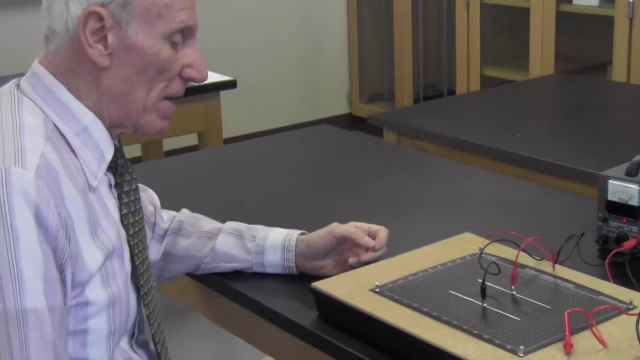 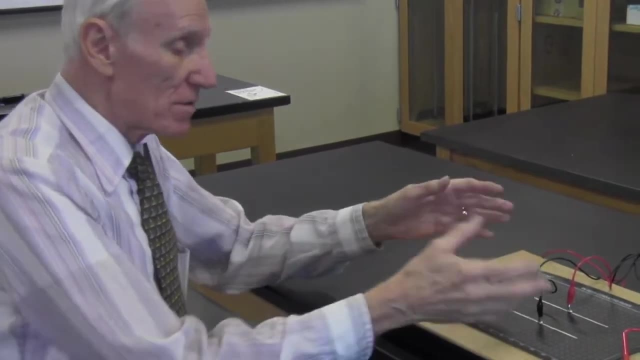 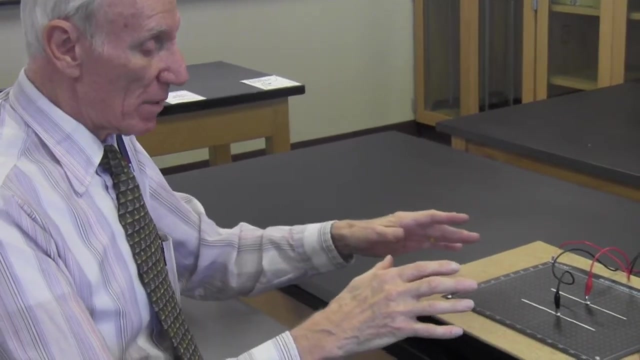 Especially for the circles. it's going to be a little bit more tricky, And then we will take a photocopy of this so that you can work on this, do any analysis without smudging up all your lines, And so we'll, at that point, when you're done with both copies or if there's time, 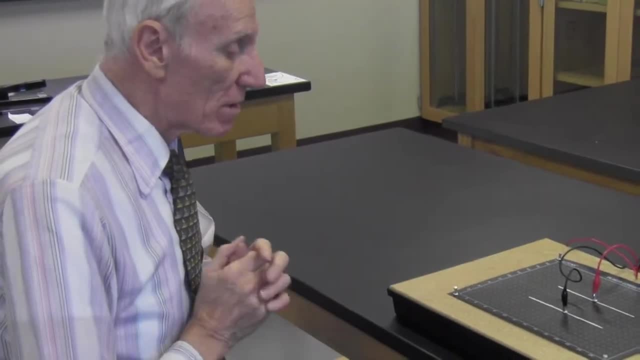 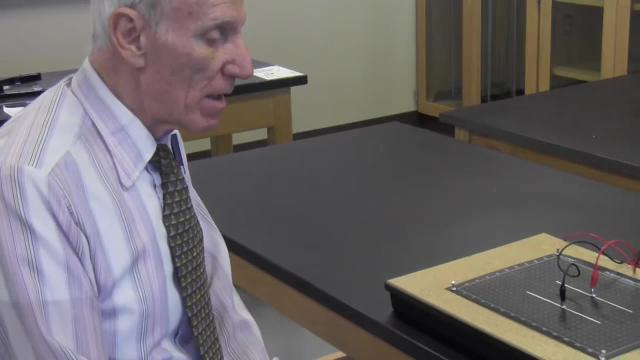 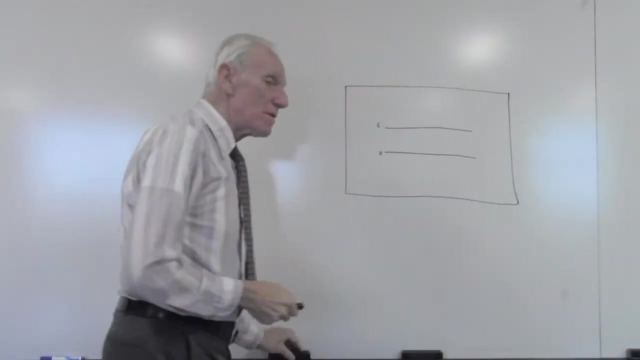 in between, if you're done with one copy, we will run out and make photocopies for you so that you can work on them without smudging things. Okay, that's it. it's a pretty simple lab. So, analyzing this again, it's a. it's a semi-quantitative, you can't do as like. 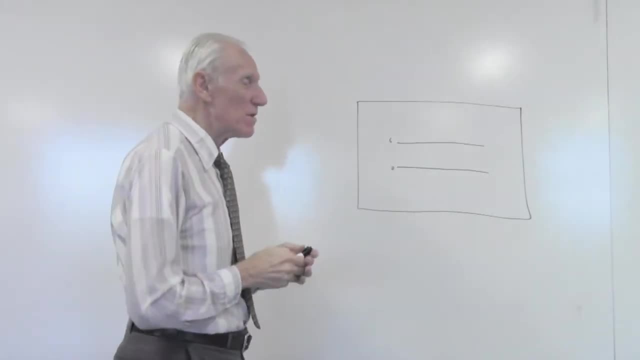 a 4% error to 1.3% or something like that, and that's kind of crazy. You can do. you can do a discussion of the error and so forth, because we always like to do that. Okay, so this is six. this is zero-volt equal potential line. this is a six-volt equal potential. 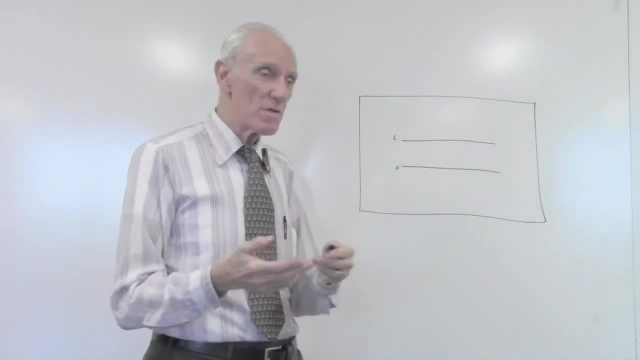 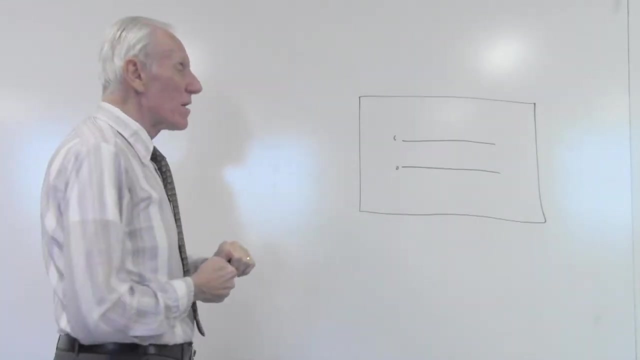 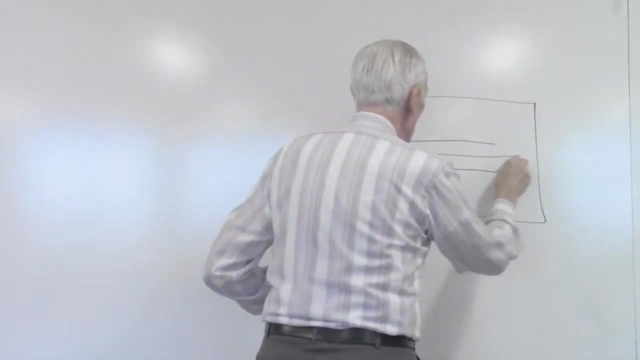 line. Equal potential means it's at the same voltage. voltage and potential are very closely related, So let me just make up what it kind of looks like, based on what you saw me do just a bit ago. So the three-volt line probably goes pretty much straight through. Well, it depends on. 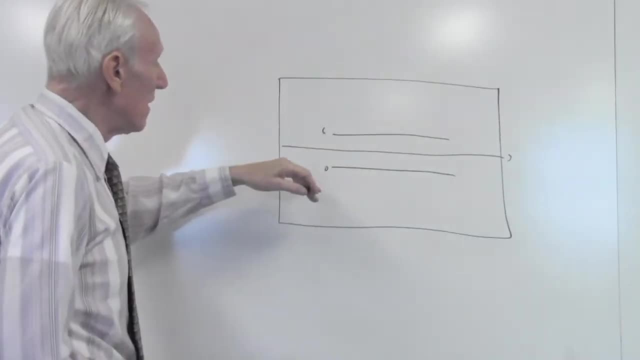 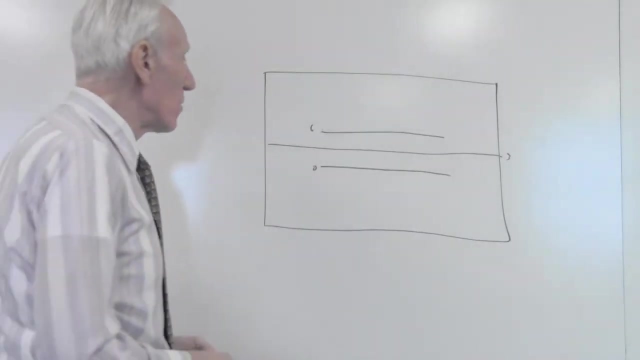 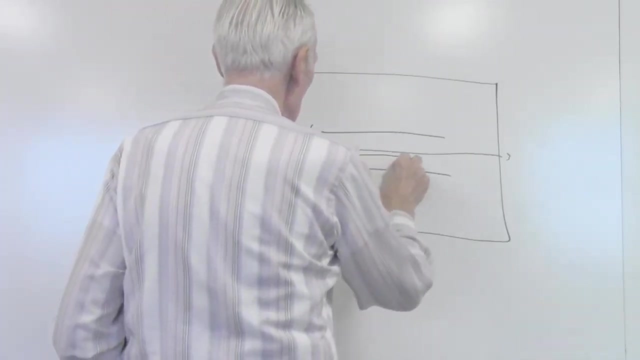 the quality of the paper and the quality of these two lines and the evenness of the graphite on the paper and so forth. So there's there's a lot of variables here. So let's look at the two-volt line. You saw the two-volt line was doing something like this. All right, 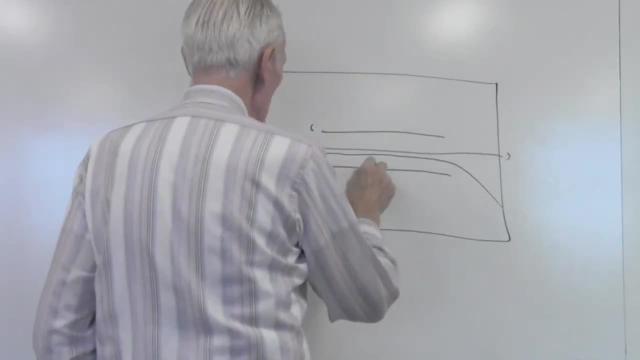 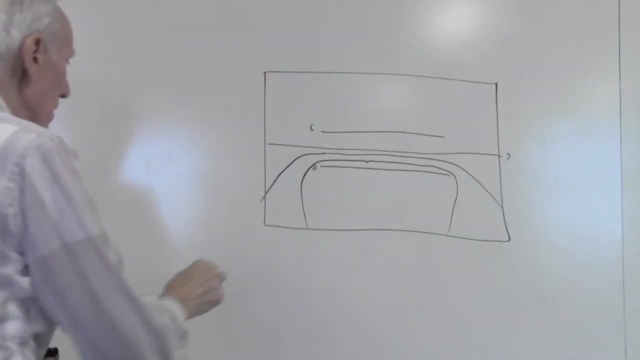 and you also saw the one-volt line. if you remember my drawing, my probing around, poking for it, it looked something like this and something like this: This is the one-volt, that's the two-volt And there's the four- and the five-volt. They pretty much look like: 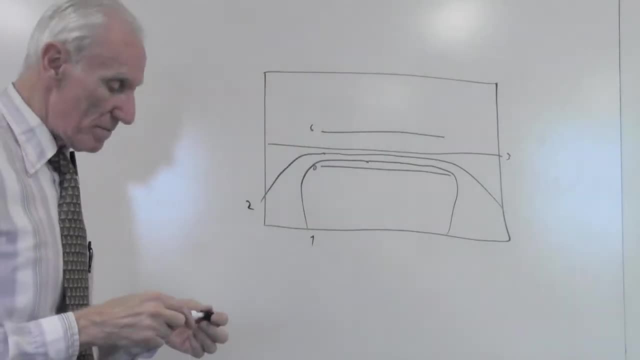 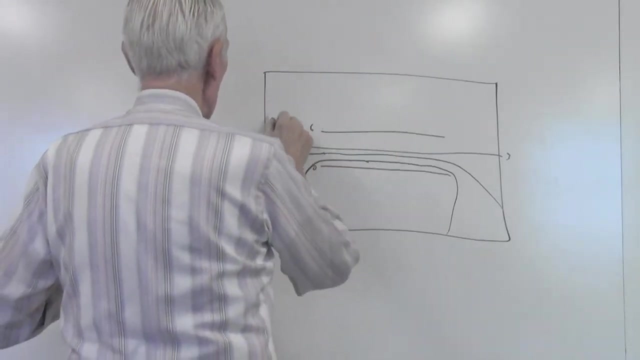 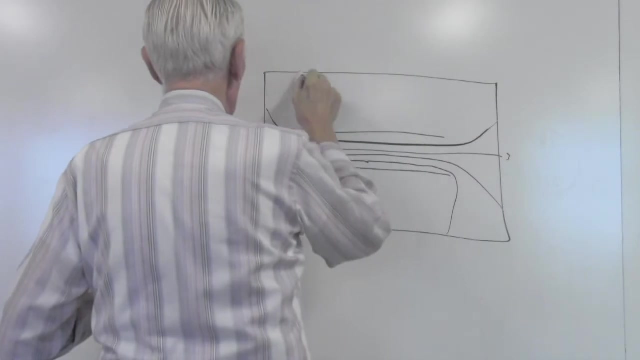 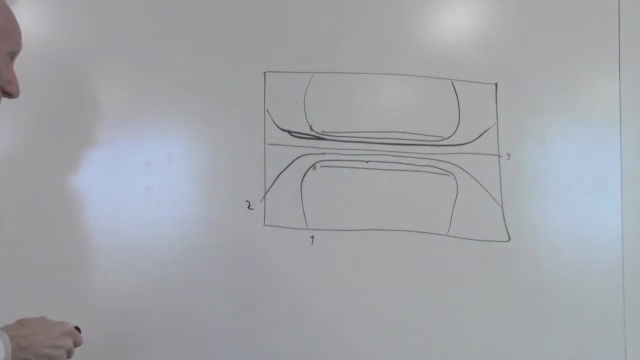 the flip side, literally, of this pattern here. So let's just, I'm going to fake this pattern, so it's going to look something like this: Oops, something like that. That's kind of what you're going to look like, Okay, so 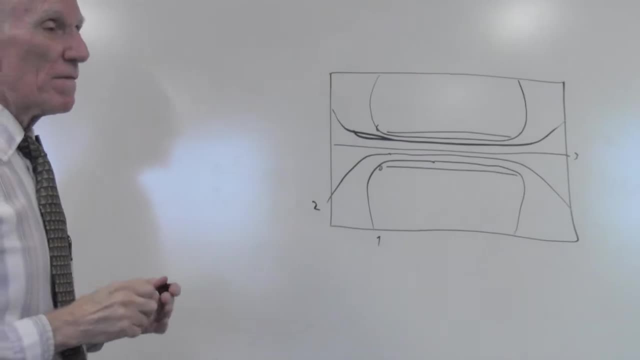 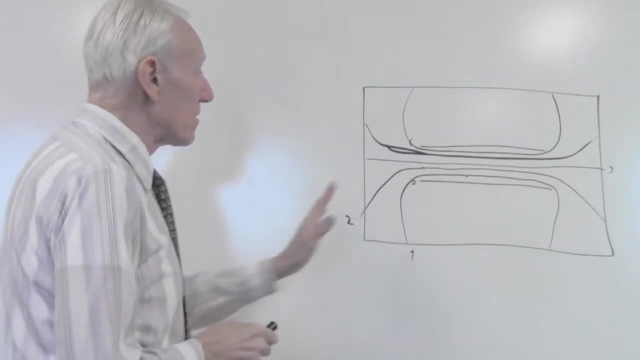 you see a lot of symmetry here, so I'm going to save you 50% of the time at least, or maybe 75% of the time if you're lucky, because there's a lot of symmetry here And it's not the same exactly as it is down here, and so if 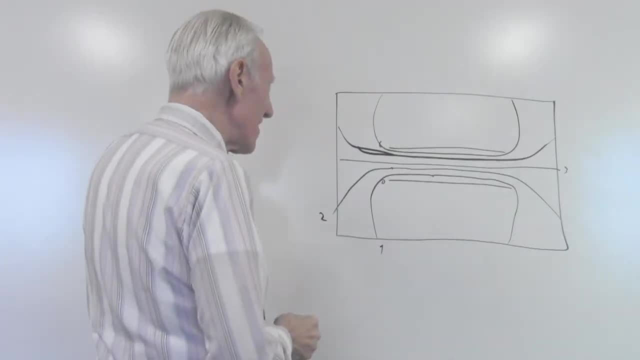 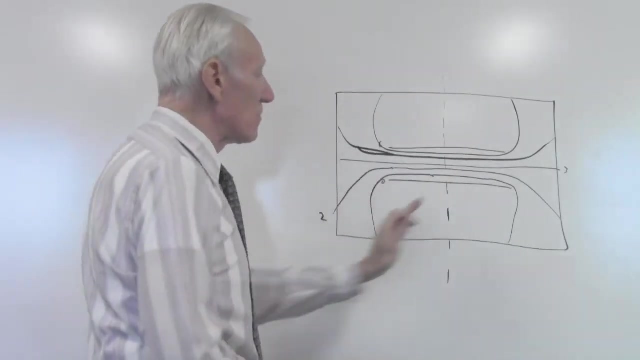 your pattern is not quite the same, you might have to say, well, okay, this side and this side are the same. so I'm going to, in my mind, just analyze one side or the other And that's enough, because this side and that side are pretty much doing the 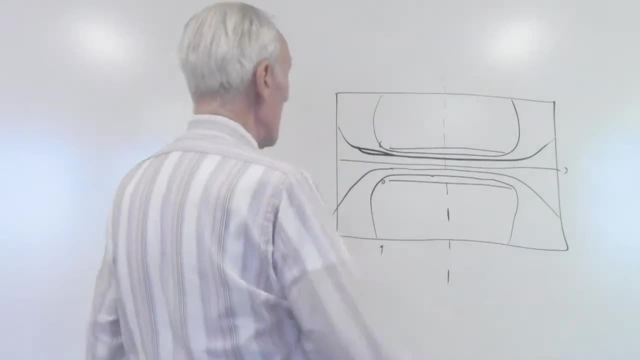 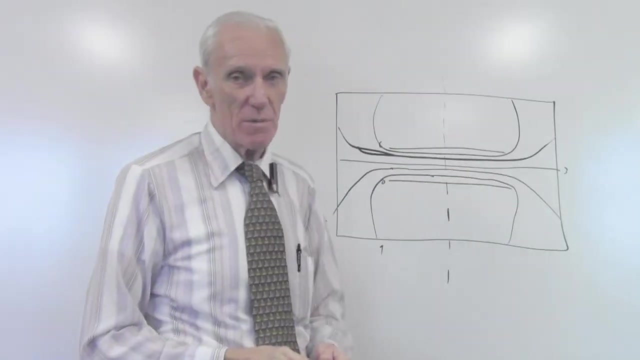 same thing. And if it's really super symmetric- like this is almost symmetric- then you can say: well, I'm just going to analyze one quarter of it, because all these quarters are the same or pretty close to the same. Again, this is a 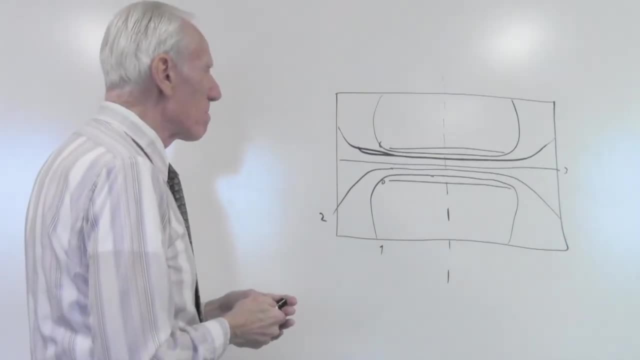 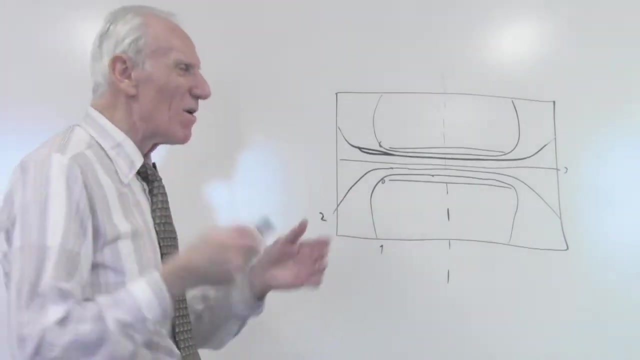 semi-quantitative law. So you know we're not going to get all hung up over numbers. This is at 0.6, is that 0.7?? No, we're not going to get hung up on that. So this is a 4-volt. 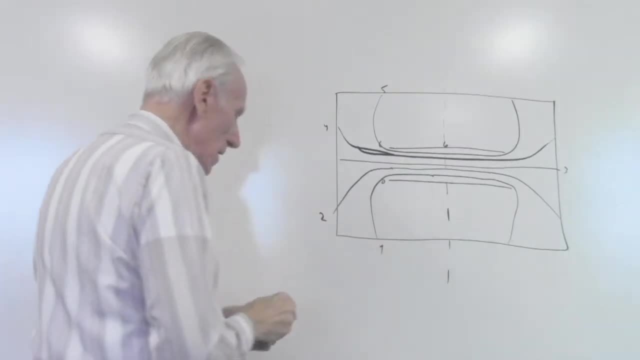 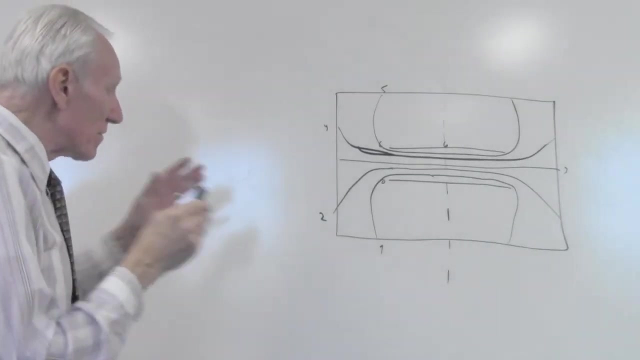 line and a 5-volt line and a 6-volt line. Okay, so that's what your pattern is going to look like. I shouldn't give away the answer, but there it is, But you've got to do it. Okay, so we have these equal potential lines. Now the nice. 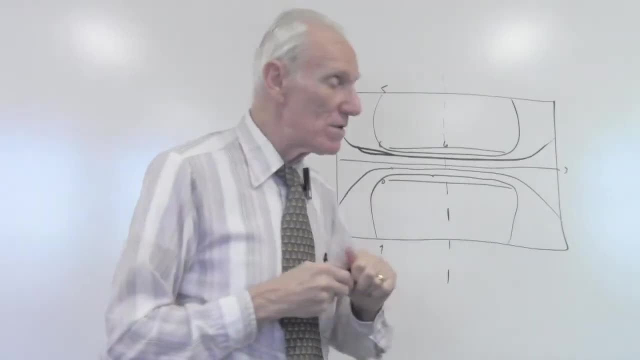 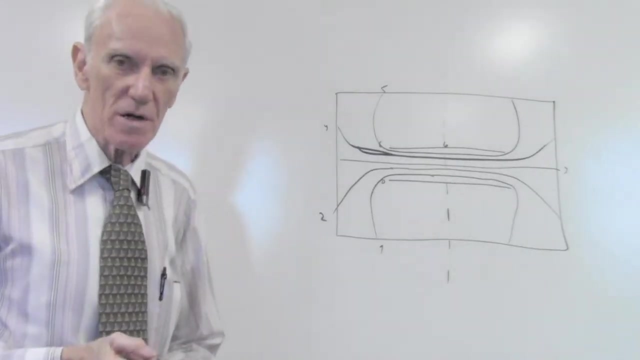 thing about fields – we have to thank the English for doing this – is that you can look at this and see already, maybe, where the field is stronger and where it's weaker. So where do you think it's stronger and where do you think it's? 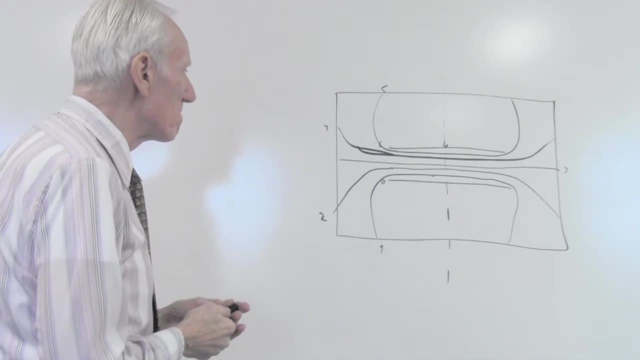 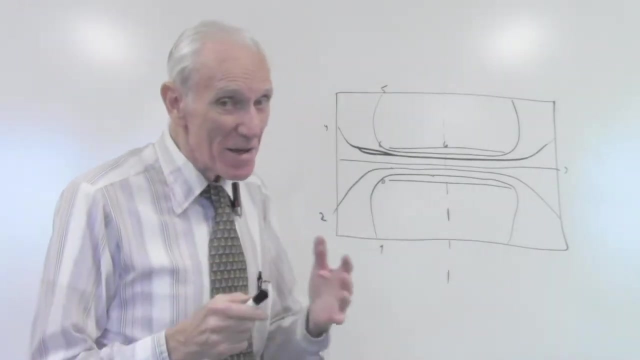 weaker. I'll give you a second to think about that. Okay, time's up. I think you can see – I think just by looking- that the field is pretty strong in here and it's getting weaker and weaker and then you get a strong field and a strong field, and that's a change from the old pattern. So have a good. 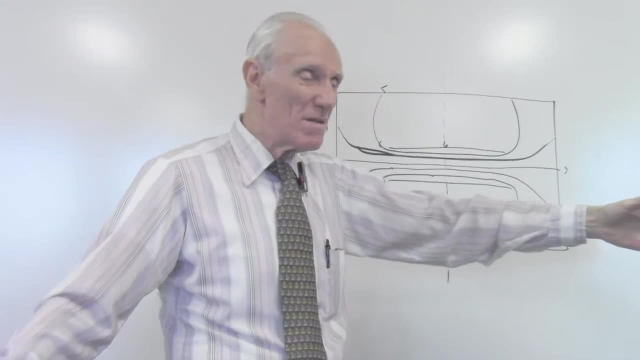 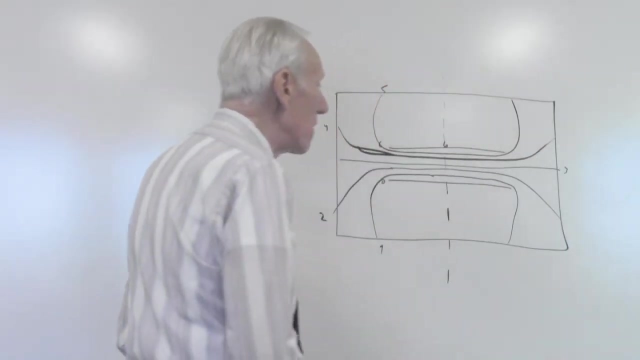 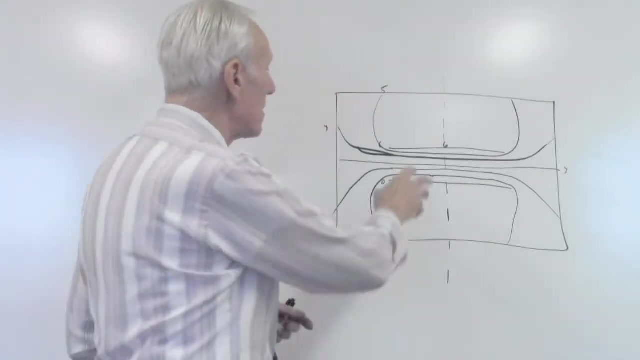 out here. It doesn't go as 1 over r squared, but it gets weaker. Here the lines are not diverging like the spokes in the wheel, but they're spreading out here. Okay, So you can look at this and see where the field's strong and where it's weak. You can see sort of the. 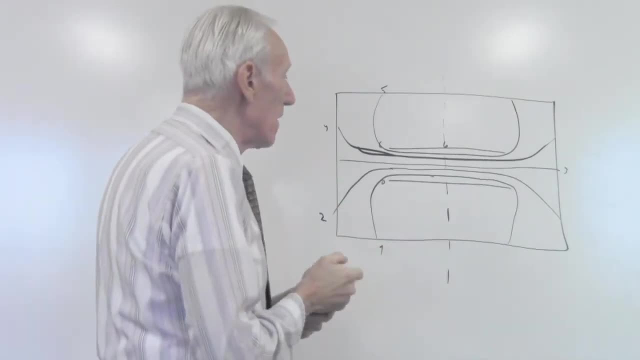 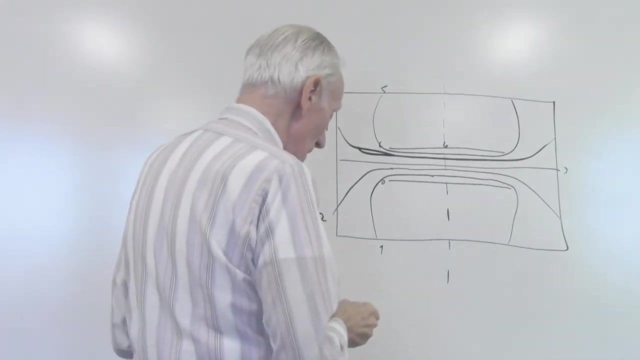 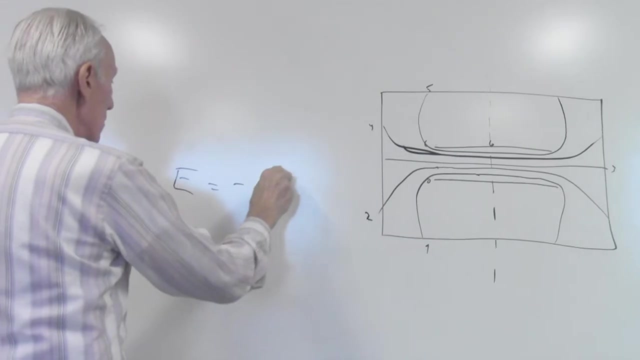 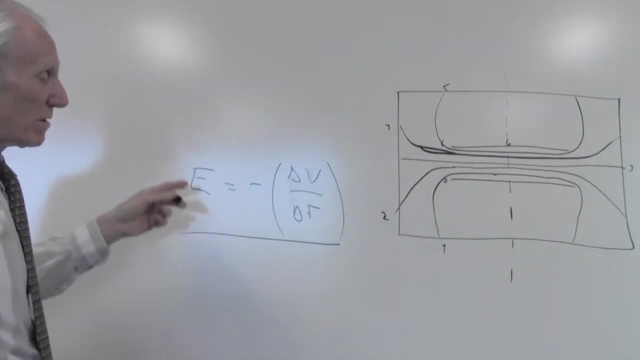 density of these lines. Better yet, I'm going to say how fast the lines are changing, with distance, For instance. okay, so here's a definition. Here's how the electric field is related to. this is an equation that you'll be dealing with in a few chapters, but it explains. 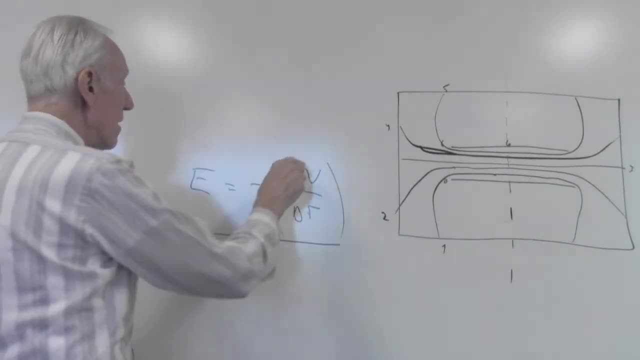 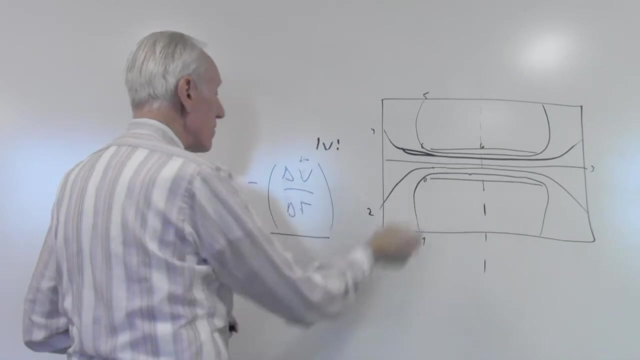 what's going on here, if you understand what this is. So here delta V is always 1 volt, because zero, 2 from 1, 1 from zero, 2 from 1, and so forth. All these are all 1 volt apart. So the difference. 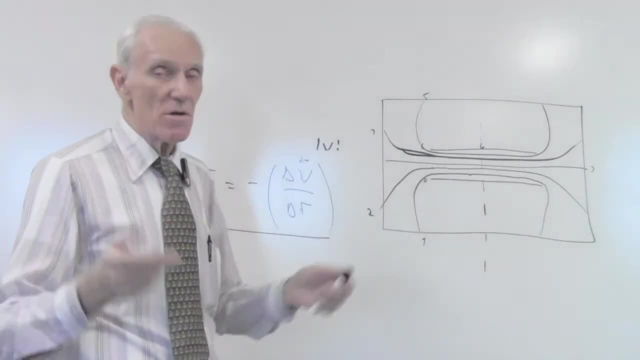 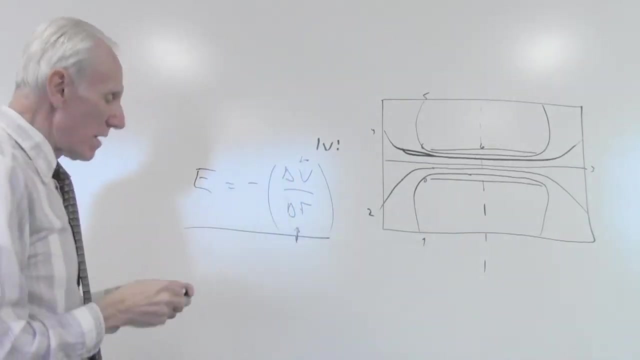 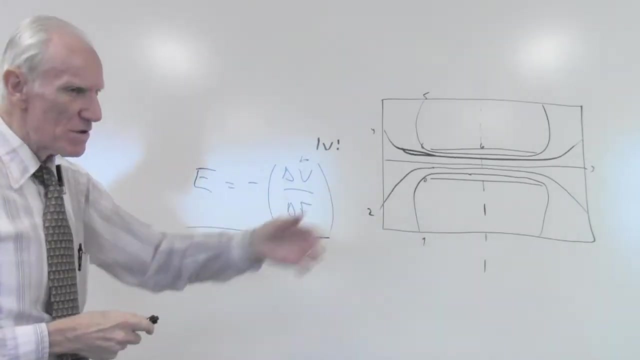 in the voltage between one line and the next line is always 1 volt, So it's always going to be 1.. And here delta r we've got to talk about that. Delta r is some kind of a distance right or a change in position. Delta means a change, r means position, change in position. 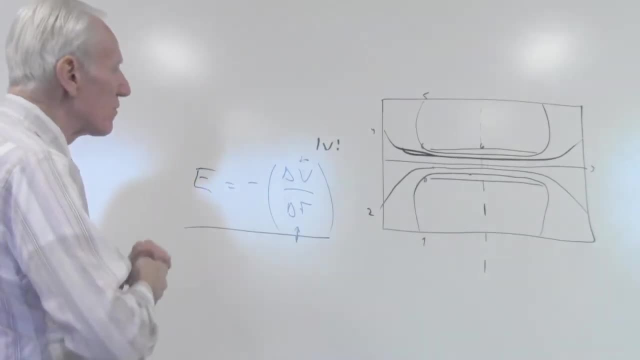 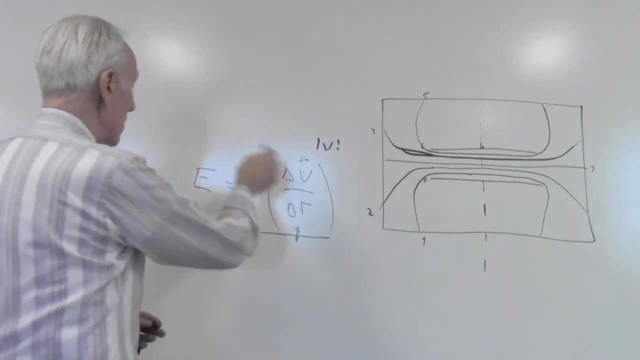 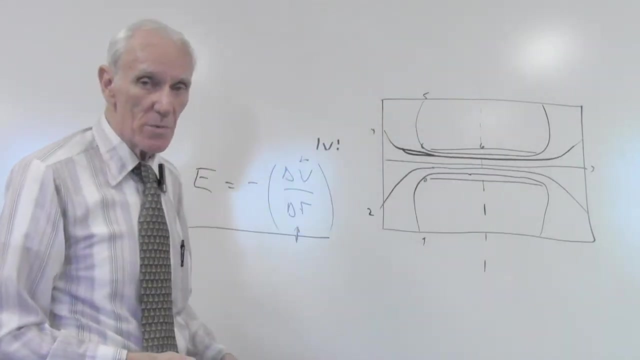 So what do we do here? Well, here's what you've got. You've got to do. this is your challenge. Once you get this pattern, you've got to figure out the electric field everywhere in half or a quarter of this piece of paper. Okay, 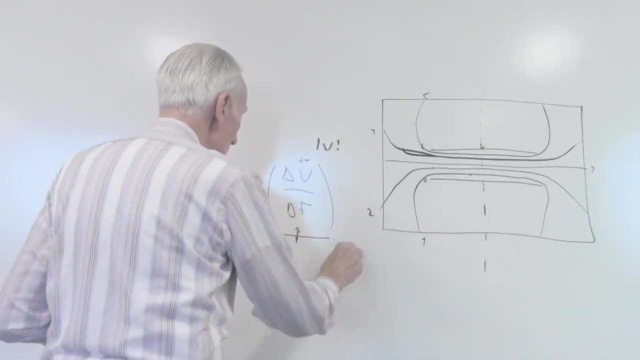 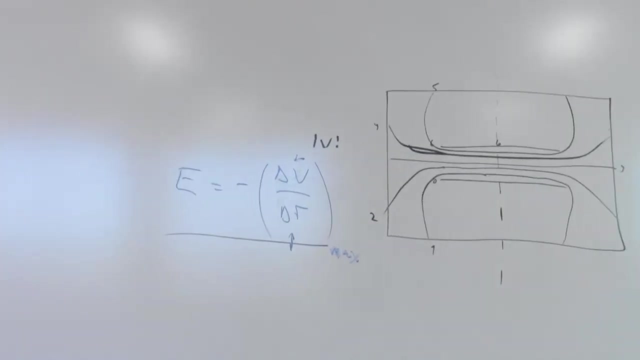 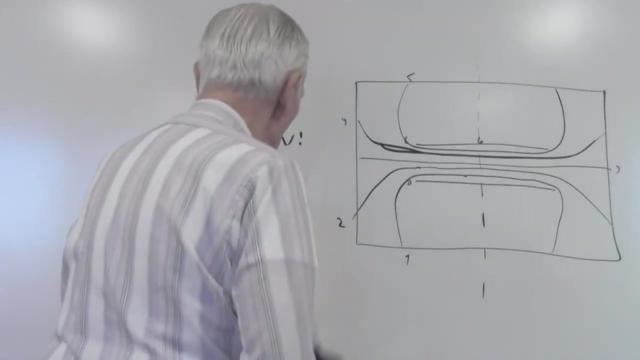 So there's, let me get another pen, Okay, Okay. Okay, Give me your pen and wake it up, Okay. So I'm going to put a little max down here. I know max is a student in one of my labs. 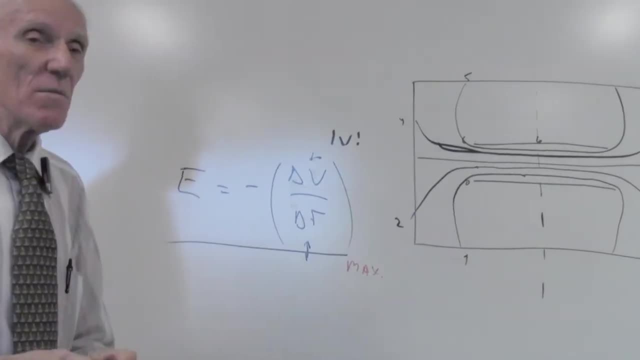 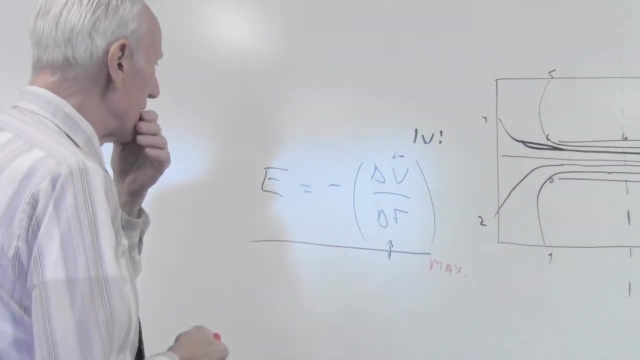 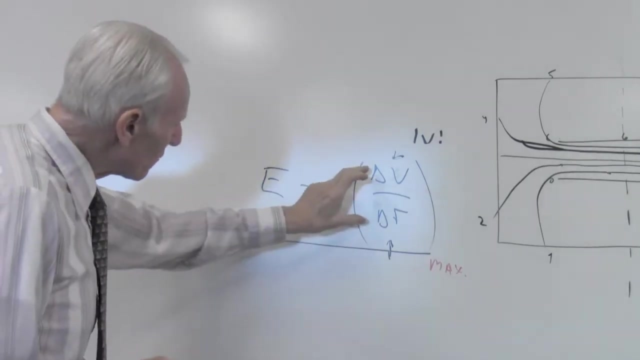 but that's okay. max max means maximum as opposed to max million. Okay, so what do they put that there for? Well, this is where you're going to have to wait for a while to get this figured out. So this expression here is called a gradient. 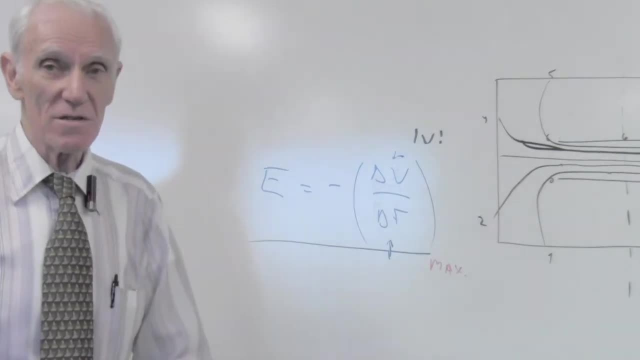 gradient. How something changes with distance is a gradient Like if you're going up a hill, you're getting higher and higher with your steps. So if you have a hill you're going up like this and a hill you're going up like this. this hill has a bigger gradient than 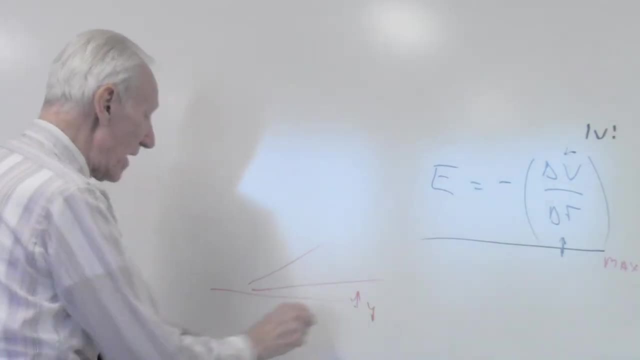 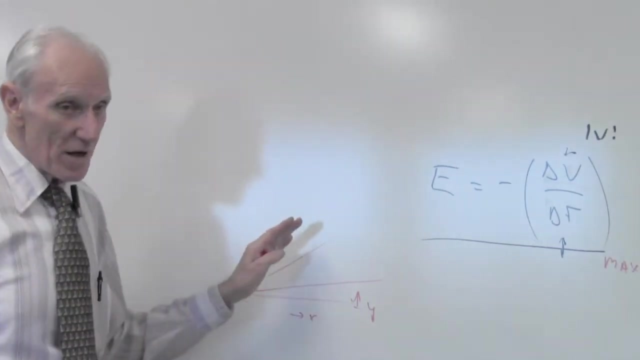 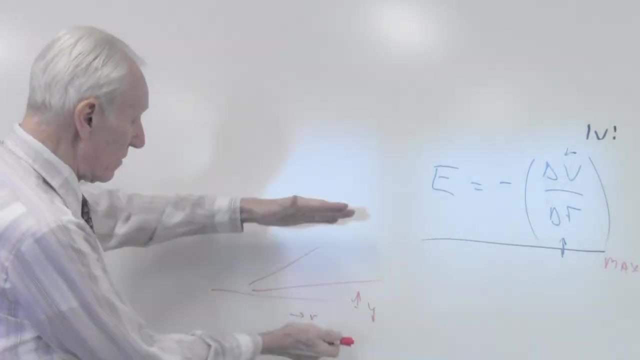 that hill because you're changing your height faster with distance here than you are here. So this has a steeper gradient. When they build interstates they try to keep the gradients to a six percent. That is a six, six this way, 100 that way, six percent gradient. So 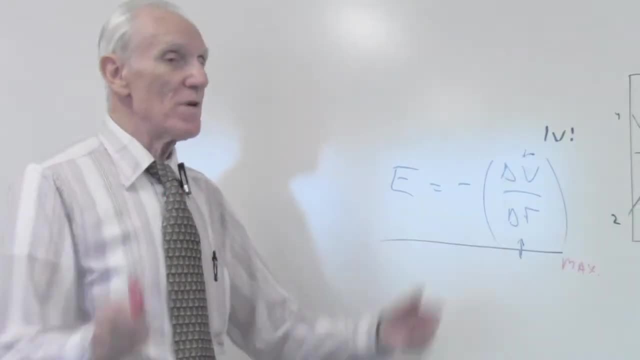 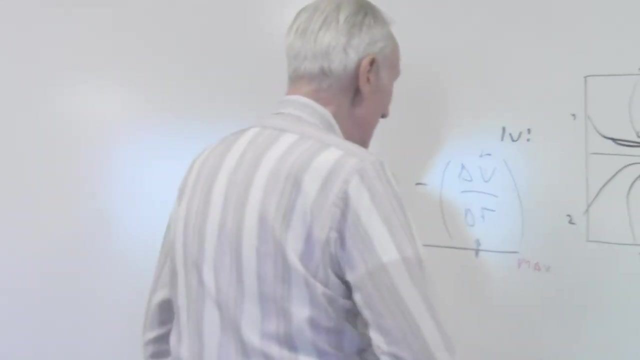 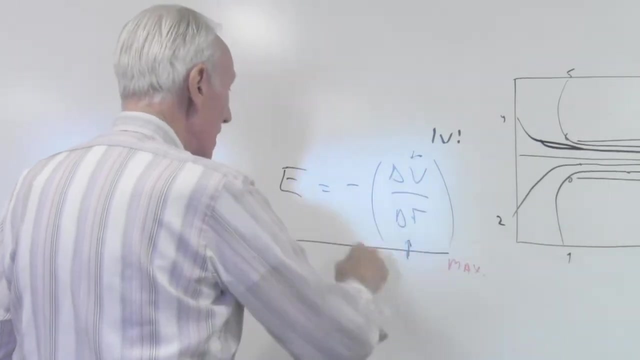 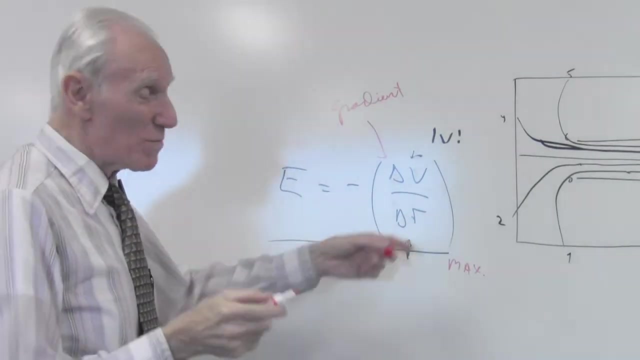 your cruise control doesn't automatically have to shift up and down all the time, Whatever. That's not the real reason. So that's what the that's what the real reason is. This is: this is a gradient. It's called a spatial gradient because it has to do with 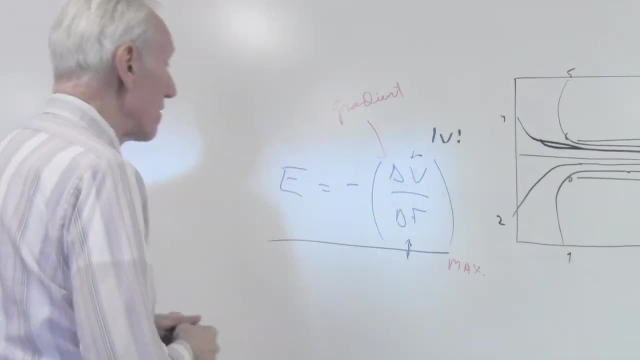 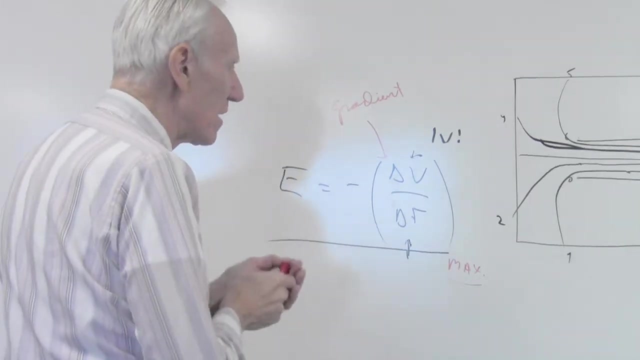 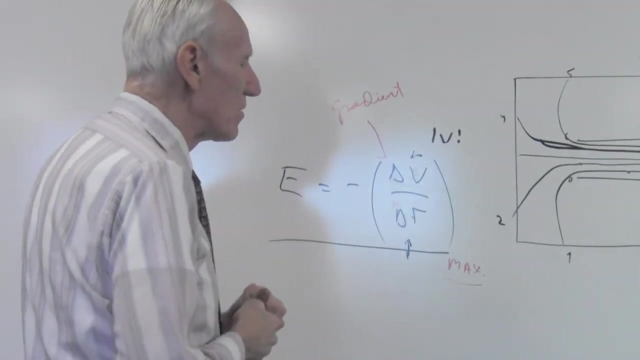 space or position, Or you can call it a voltage gradient if you want. voltage with position, Okay. so why do I put this max here? It's because you'll learn in chapter 24 or when you get to whatever book you might be looking at, when you get to electric potentials, which 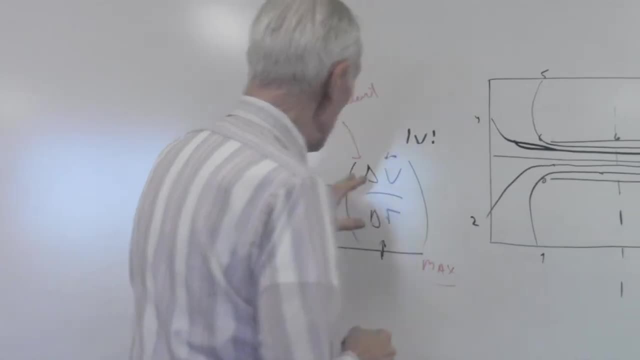 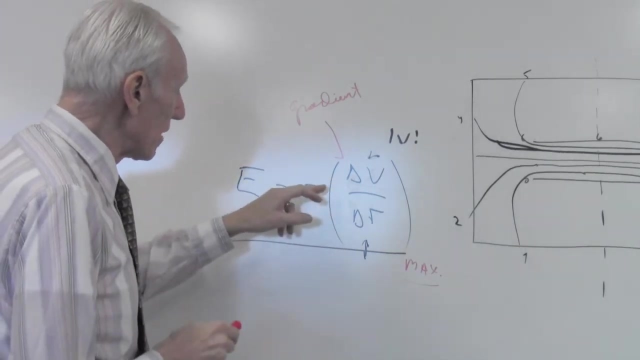 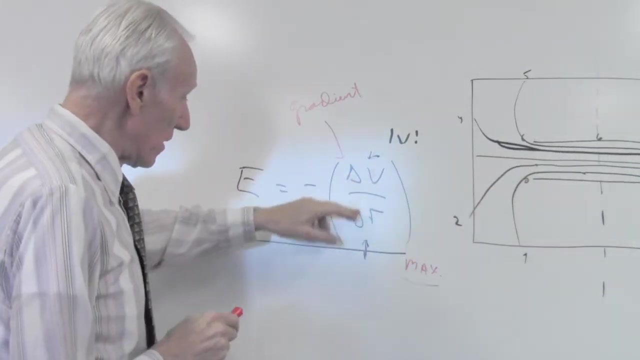 is what we're talking about. You see, we have the fact that the electric field is in the negative direction- we'll talk about that in a minute. in the negative direction of the direction which the voltage- you have equal potential lines, equal voltage lines- changes the fastest with distance. 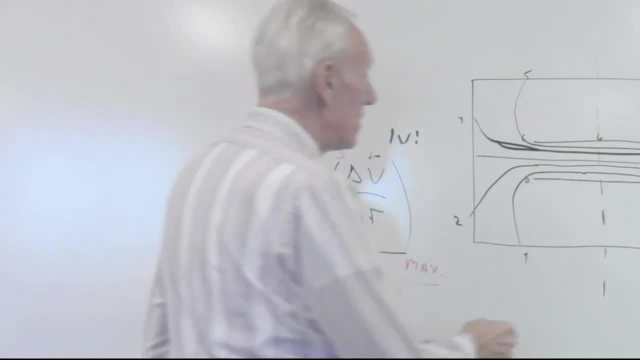 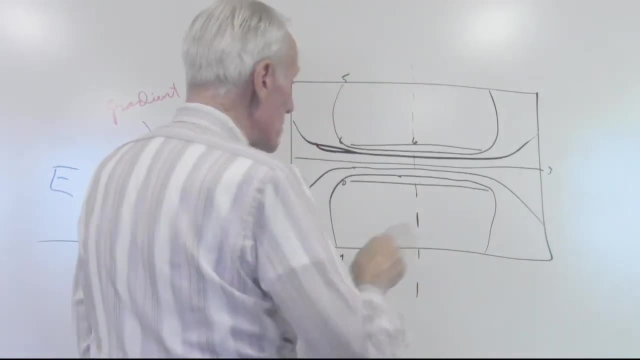 That's what that means. So if I go from, say, zero volts to one volt here, I would go from here to here. That's quite a distance, But if I go from zero volt to one volt here, that's a really short distance. In fact, the 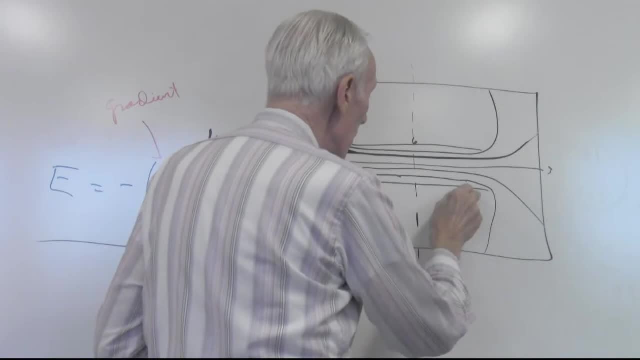 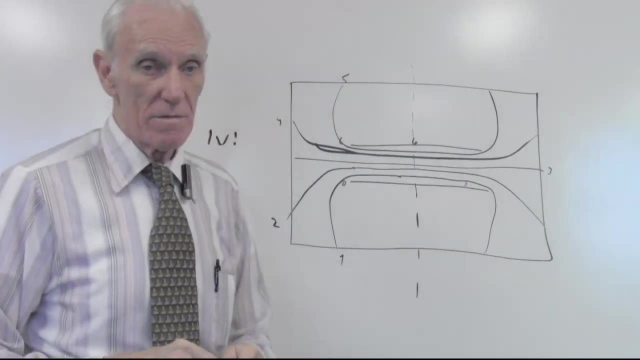 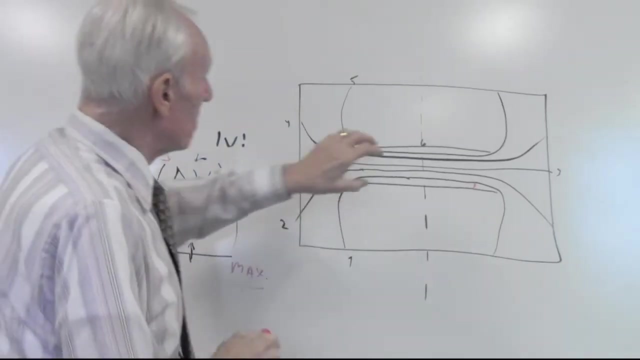 shortest distance to go from zero to one volt is where you draw a line that's perpendicular from the perpendicular from the one volt line to the zero volt line. That's what this really means. So and again, just by looking at it you can see the field is strongest here, right? 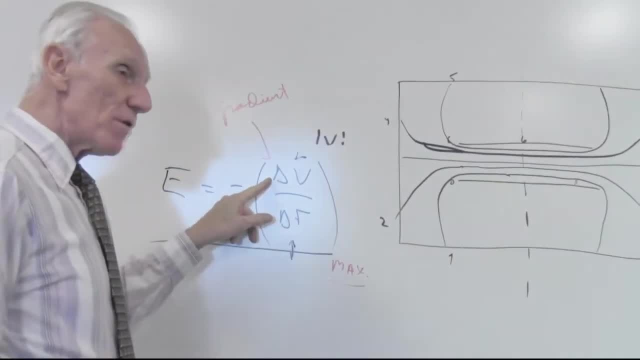 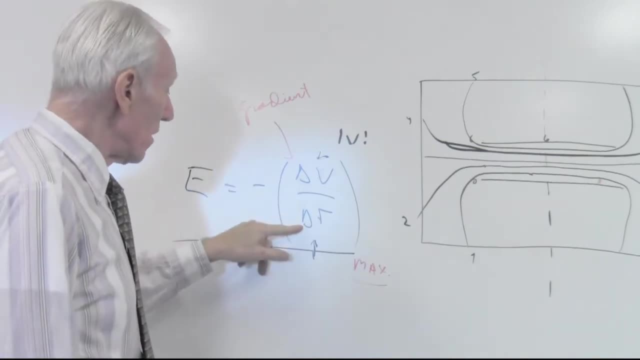 What does that mean? That means you don't go very far Before you change by one volt. So this is a small number. That's always one volt. So if that's a small number, if it's the smallest, then this number is the biggest, which is: 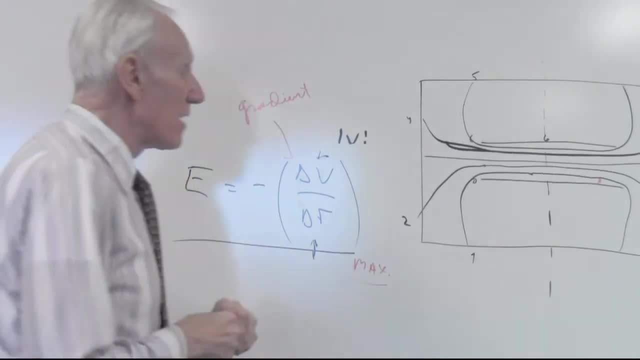 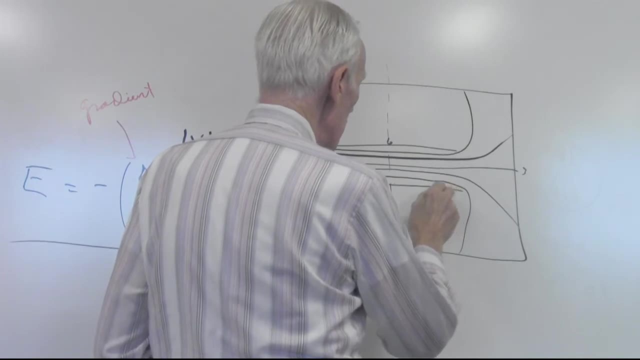 the electric field direction. So this is kind of nice. So what you do then is you have to do this: draw lines perpendicular to these. the electric field direction is in the direction perpendicular to all these lines here, So I'm going to go from here to here. 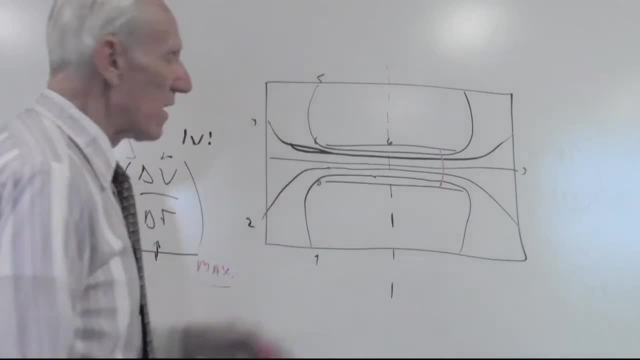 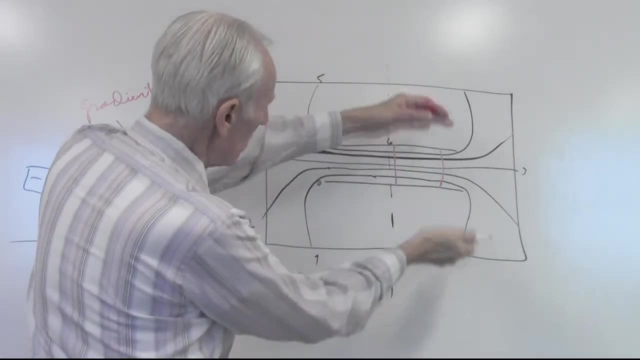 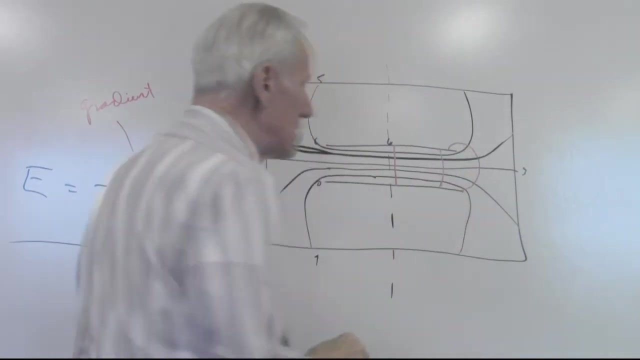 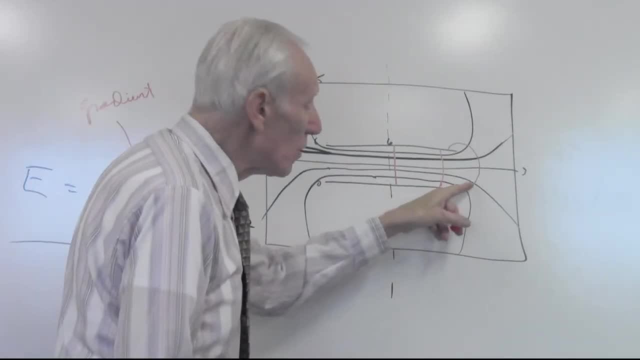 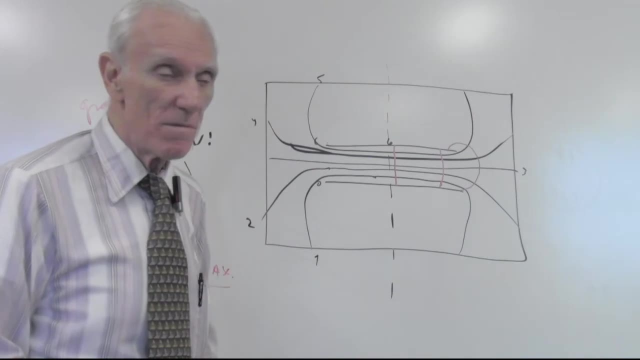 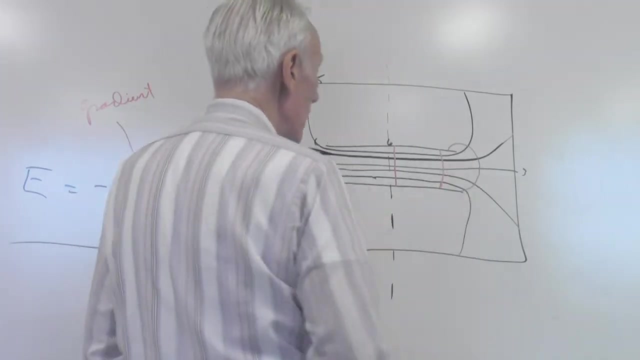 I'm hitting, I'm going across these, these equal potential lines at right angles- I didn't do such a hot job there, but at right angles to every line. So that's what this means. The shortest distance from electrically from this line to this line is perpendicular to. 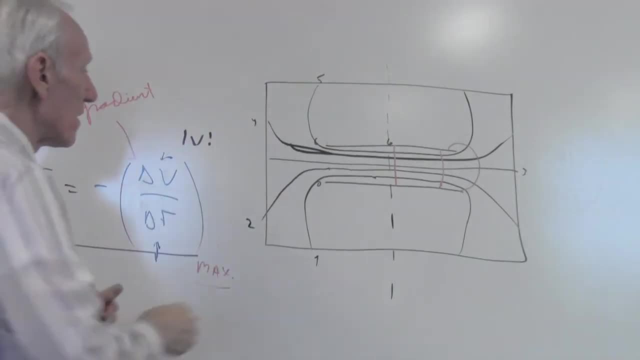 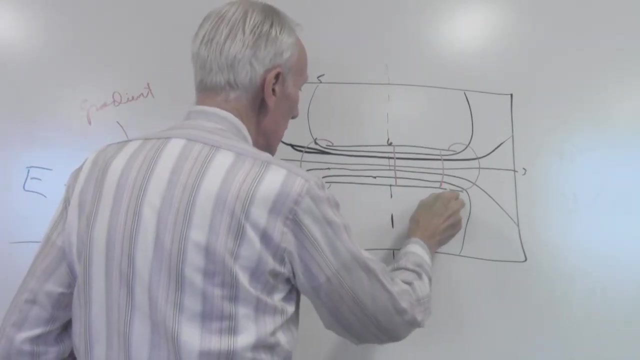 each of those lines, So those I've just drawn a picture of the electric field lines. There's another line like that over here, and so forth. There's a line like that goes, comes out here, goes, perpendicular, perpendicular. 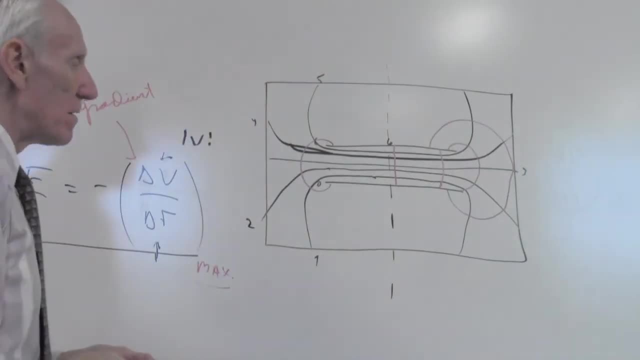 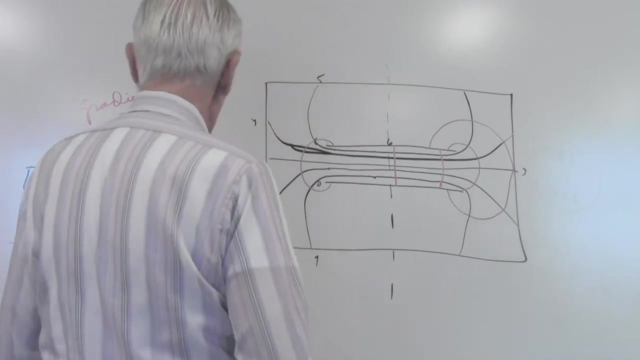 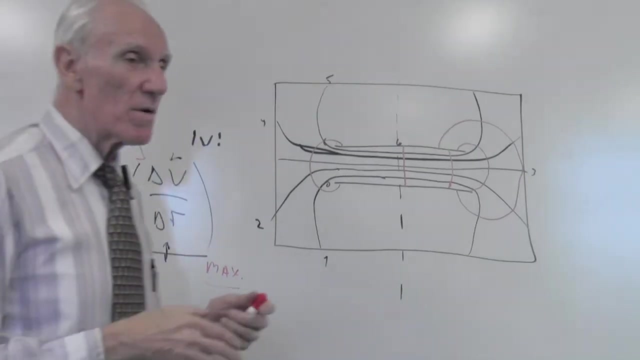 perpendicular, perpendicular and they're like that. So these are pretty arbitrary, but again they should be pretty symmetric, Okay, so again that's how I draw the field lines, And what the minus sign means is the electric fields go from a high potential to a low potential. 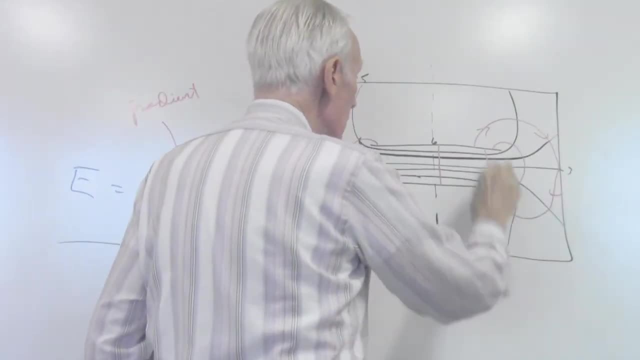 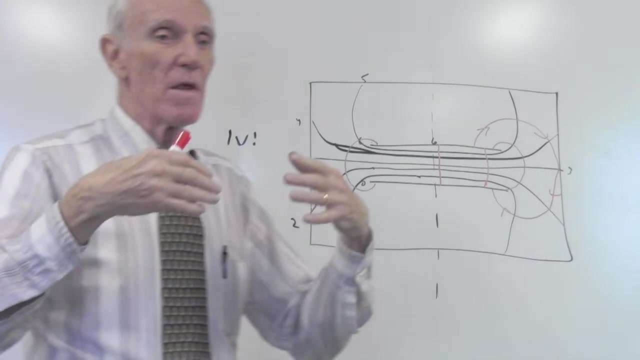 So they go this way: They go from six to zero, not zero to six. So that's what the minus sign means. The electric field is in the direction in which the potentials go down, Which kind of makes sense, I hope, And so. 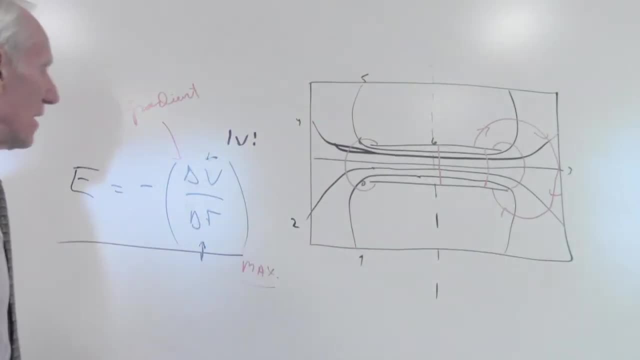 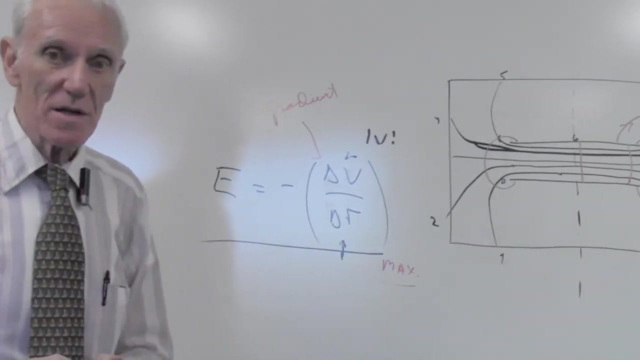 That's what the minus sign is all about. So now you know the inner workings of the chapter. on how the electric potential and electric fields are related, We know this. We're going to learn a little bit more about that in a specific later on. 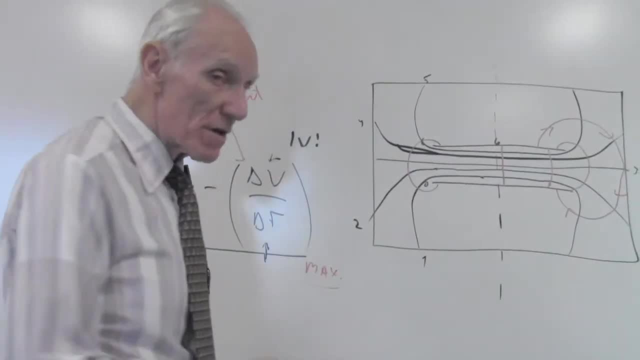 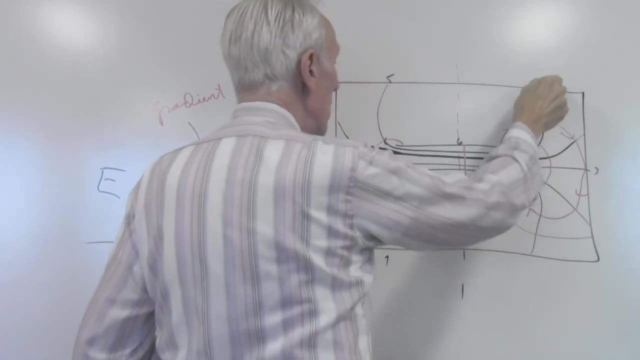 So here's this pattern. It's emerging. I'm not going to draw the whole pattern. You're going to draw the whole pattern And draw enough lines here that you fill up. there's a line that goes off the paper and comes back on over here. 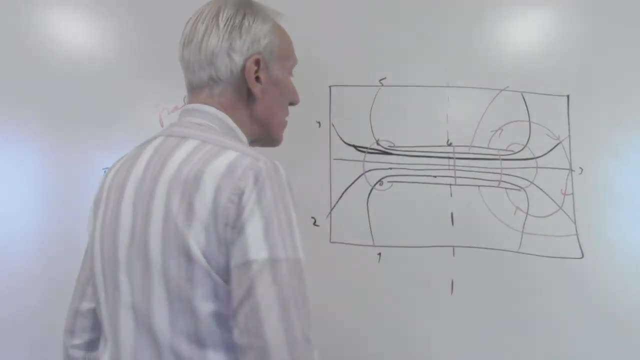 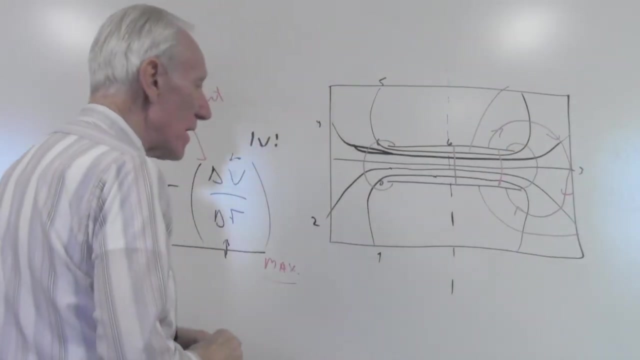 Something like that, I don't know. So you want to draw enough field lines that you have pretty much filled up this page, or half the page, or a quarter of the page, with electric field lines. Now the trouble is you've got to label this on a piece of black paper, which is tricky. 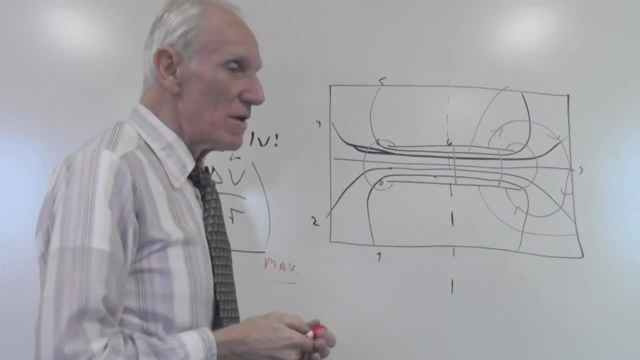 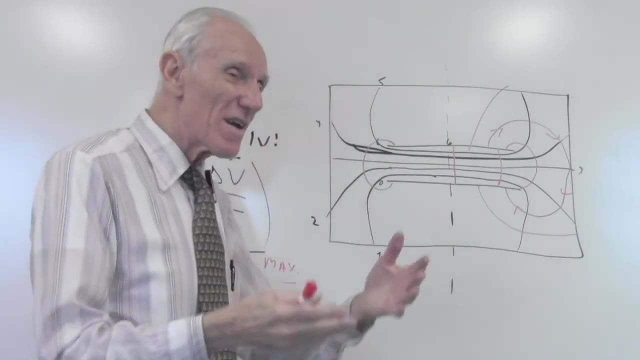 So there's all kinds of subtle ways to do that. You can use white marking, correction fluid or whatever. We'll try to copy this so it's lighter than the black paper, so that you can actually write on it And you can see what's going on. 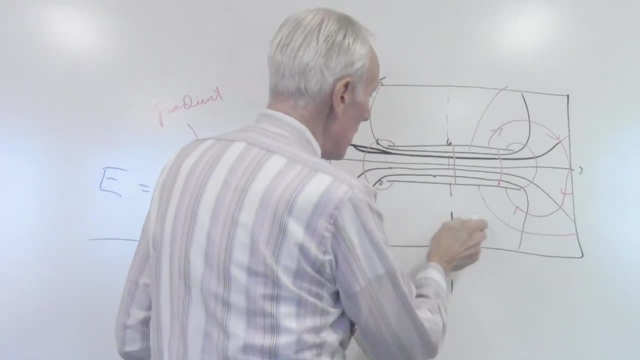 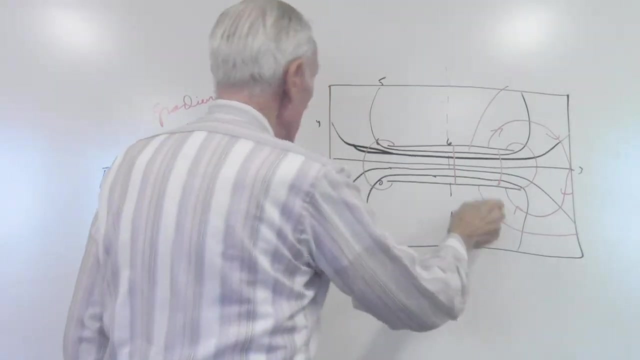 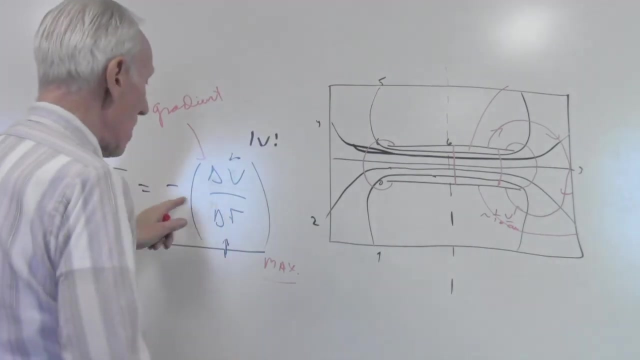 So the electric field here, let's say this, is 10 centimeters from here to here And the voltage change of course is always 1 volt. So the electric field here is about 1 tenth of a volt per centimeter. 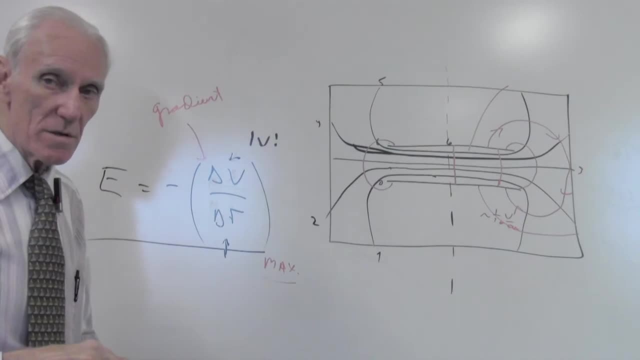 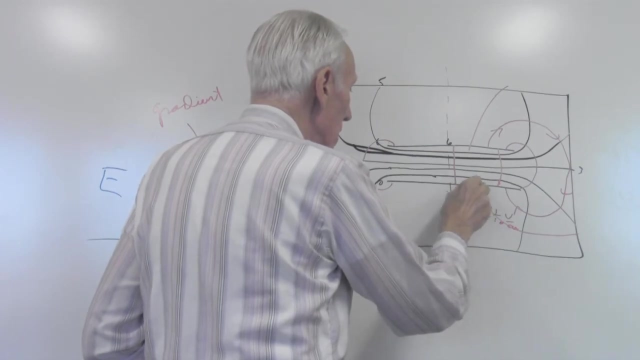 One tenth. 1 divided by 10, a tenth of a volt per centimeter, And the electric field here, as I told you earlier, is about 1 volt per centimeter, Because the lines are 1 centimeter apart and the voltage difference is 1 volt. 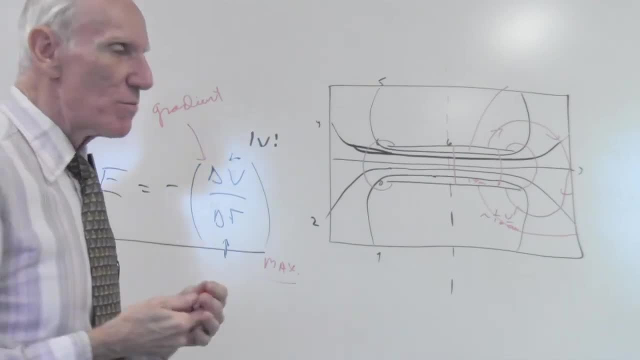 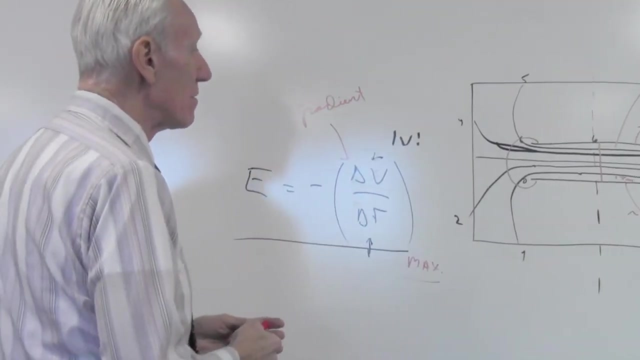 So it's pretty simple. It's kind of fun and brings back fond memories of connected dots, days in grade school and so forth. So that's the theory behind it. That's some of the theory behind it. You'll get into more theory as you get into the chapter on the electric potential difference. 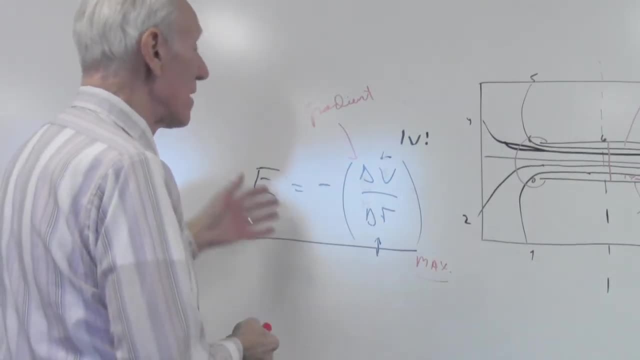 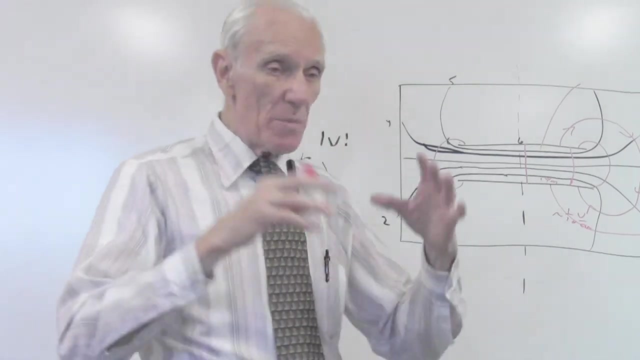 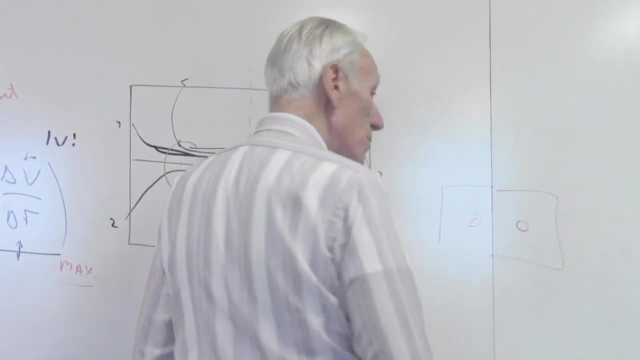 which is called voltage, And the electric field. But that's how you map out the electric field in this case. So the mapping out of the electric field with the two circles is going to be a little bit different, a little bit trickier. 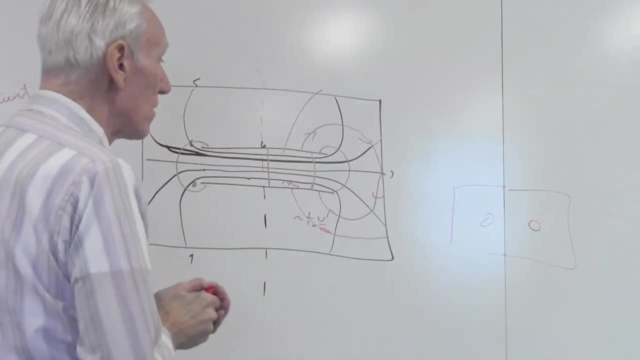 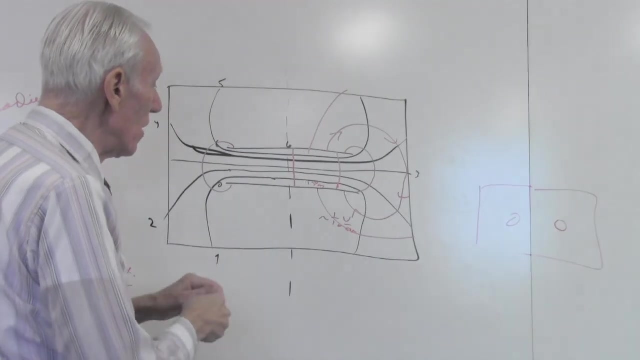 There will be lots of symmetry there too, And you can also analyze half of it or a quarter of it, And you have to somehow come up with a table that shows you Where am I talking about. So I'm going to label this A and I'm going to label this B, and I'm going to label this. 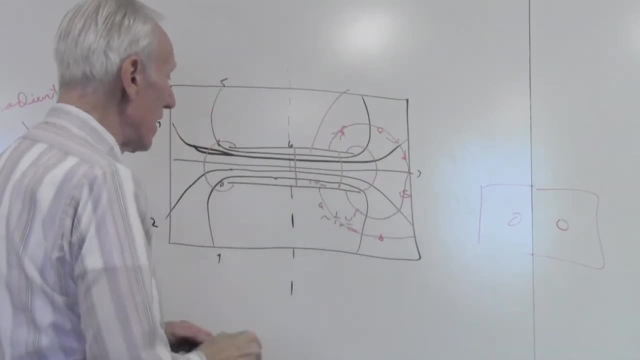 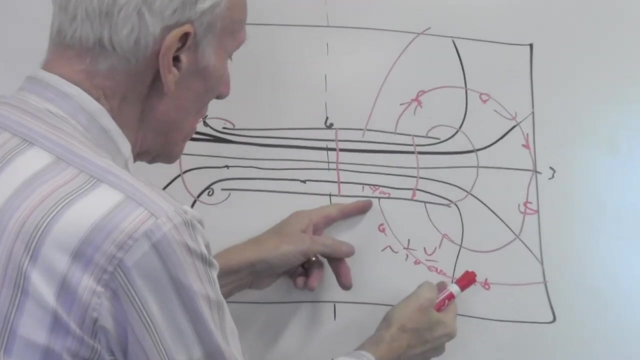 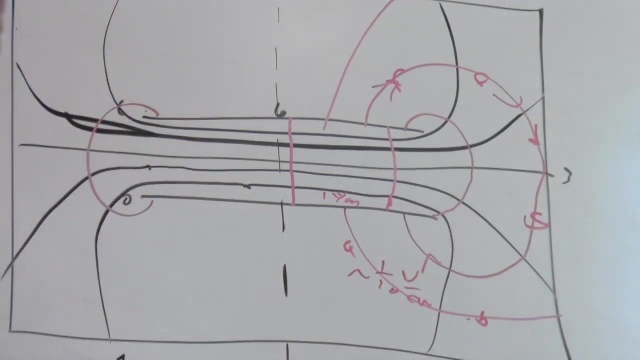 C and D and E and F or something like that, And so I'm going to run out of letters pretty quickly. So the field here is weaker than the field here. The field here is stronger than the field here because I go a shorter distance to go. 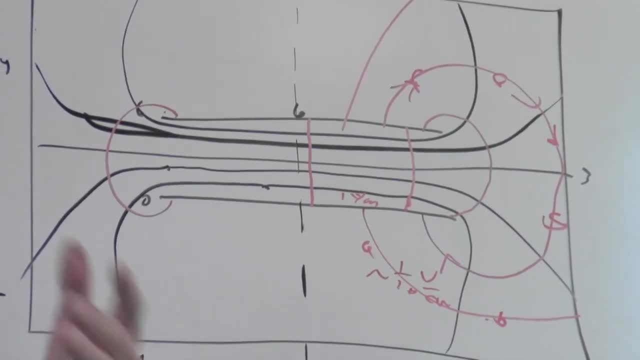 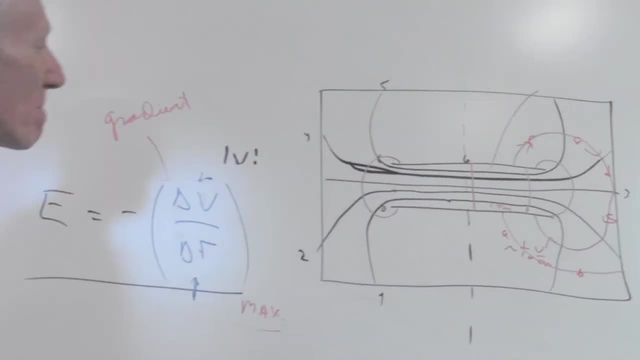 by a 1 volt change. So you can see that, You can see it coming, And so A nice visual lab for a change. OK, that's it. 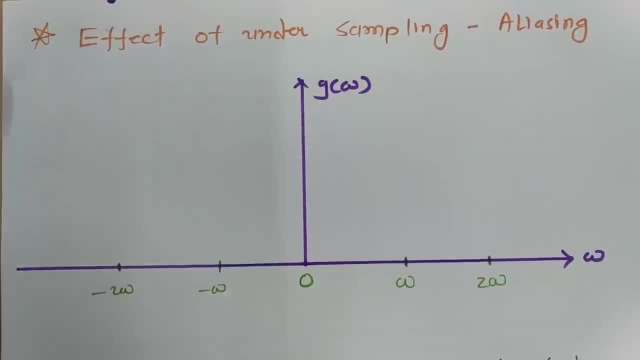 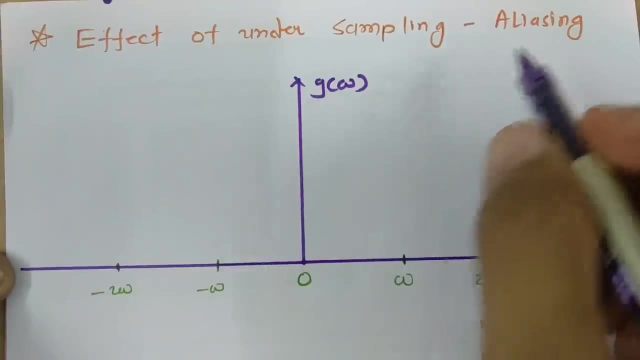 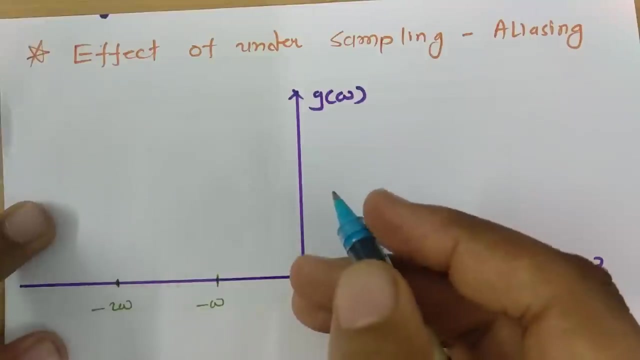 Welcome to digital communication engineering playlist. Here in this session I will be explaining effect of under sampling, that is even referred as Alloysing. Now, first of all, what is under sampling and how alloysing is happening. So to understand that, we need to see our previous session where I have explained